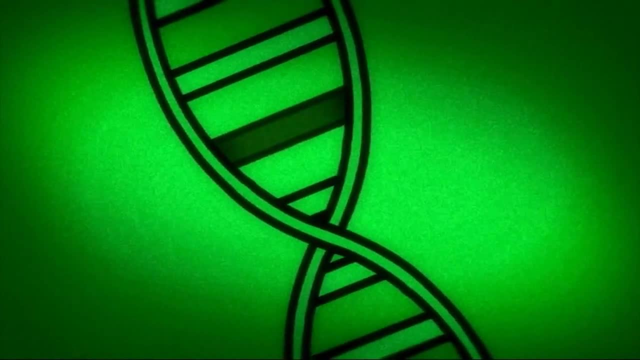 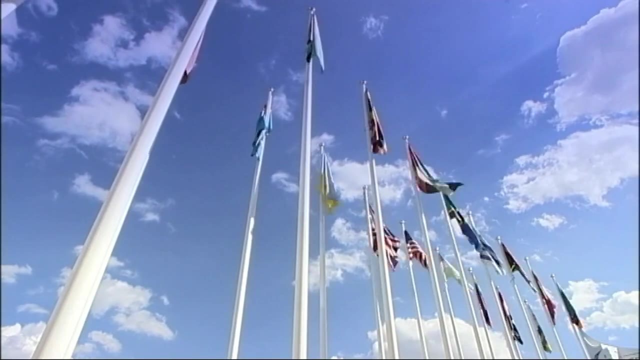 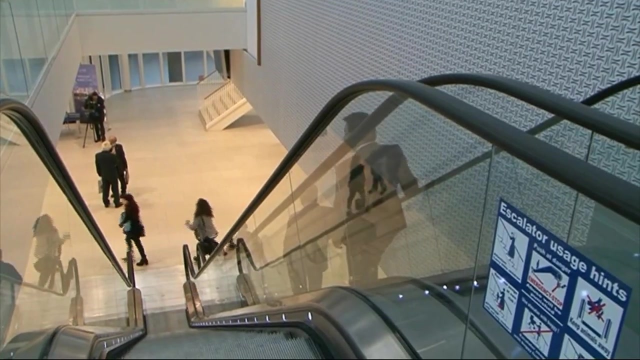 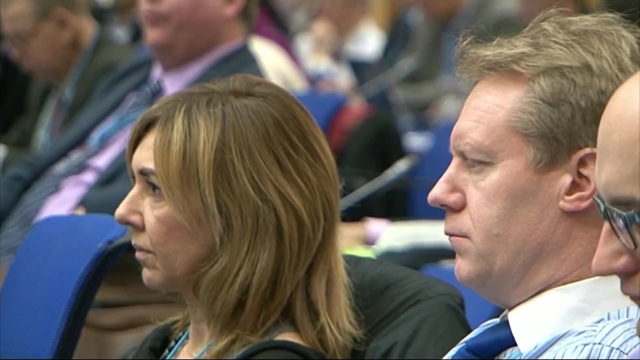 the cells that make up human organs and tissues. It can affect the DNA, which, in turn, can lead to cancer. The International Atomic Energy Agency is responsible for protecting people and the environment from the effects of this radiation. In 2014, it hosted a major conference in Vienna on occupational radiation protection: Protecting 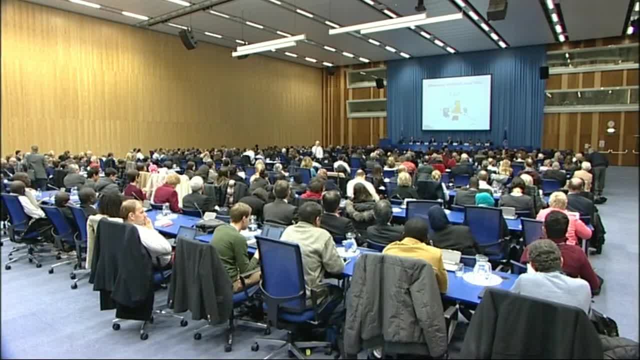 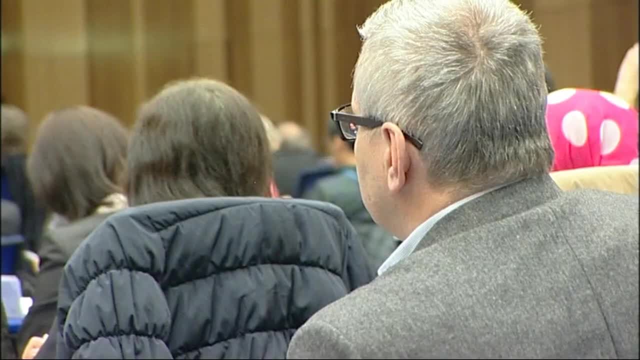 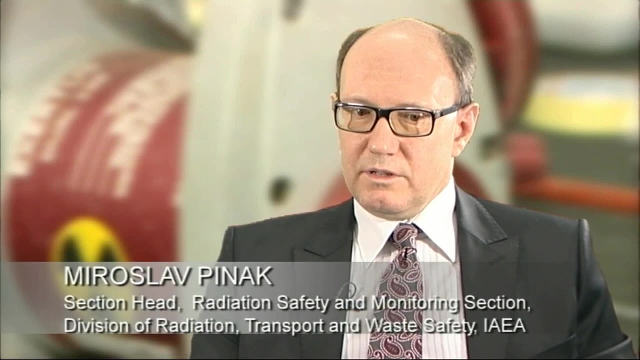 people who work with radiation work with radiation. The conference attracted delegates from all over the world. The goal to ensure adequate and satisfactory level of radiation protection around the world is a vision for all of us. Our role in radiation protection and radiation protection problem is to ensure that actually. 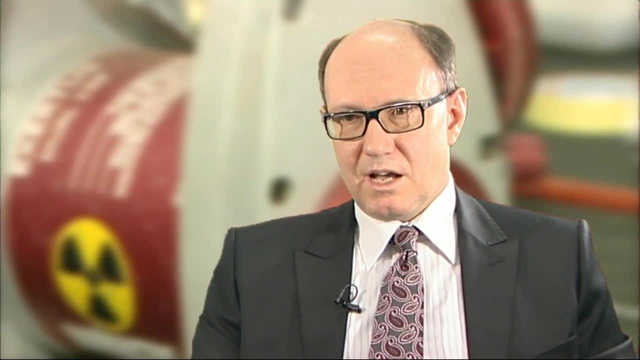 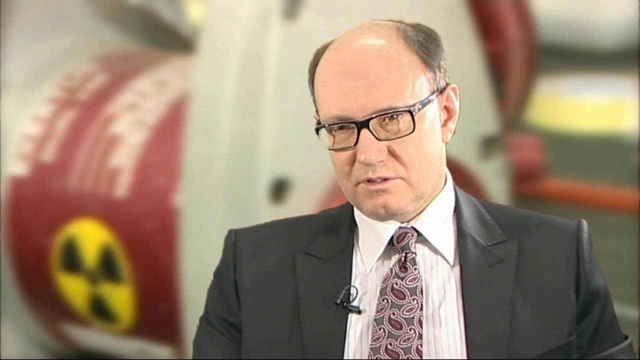 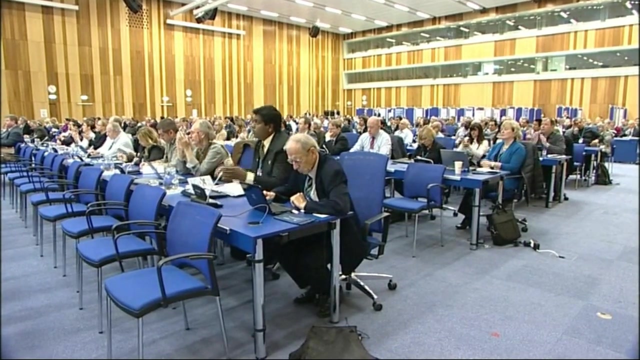 there are adequate radiation standards and guides in place which are being advocated by these member states to use and implement them in their national legislations. The Agency has a special unit devoted to protecting people who are exposed to radiation in the course of their daily work. 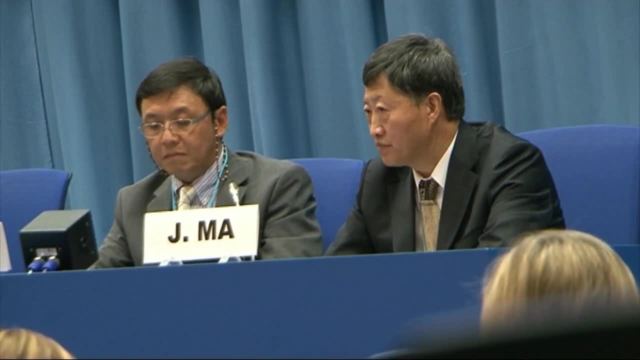 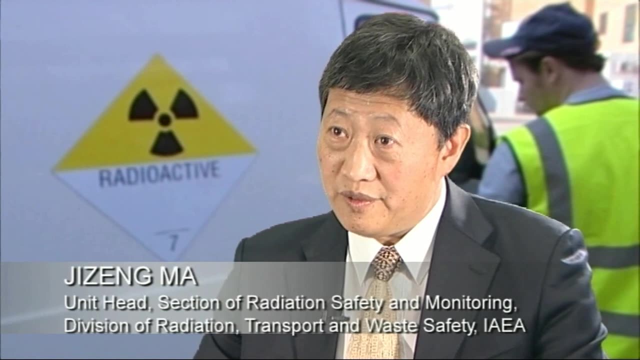 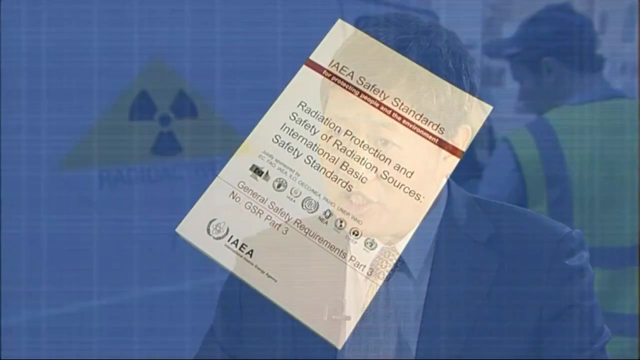 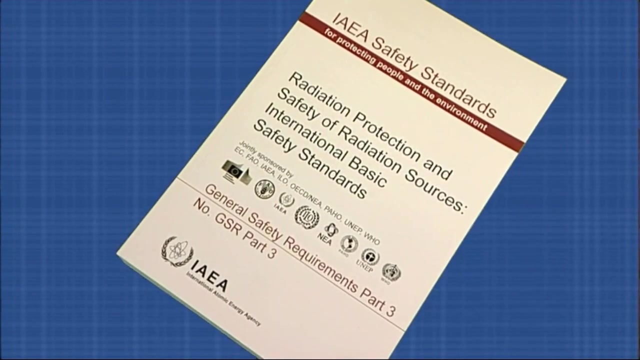 It runs the Agency's Occupational Protection Programme. In IEA we have a programme on occupational radiation protection. The project of this programme is to promote radiation protection optimisation through radiation. We are developing safety standards and guidelines with an international harmonised approach And in the meantime we provide assistance for the application of these standards and 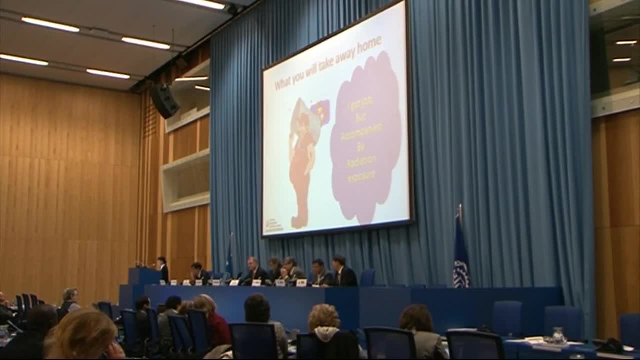 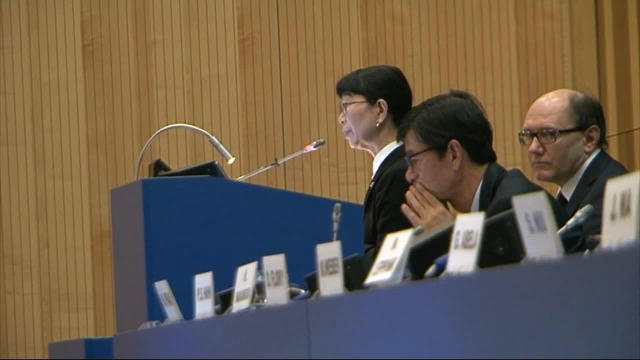 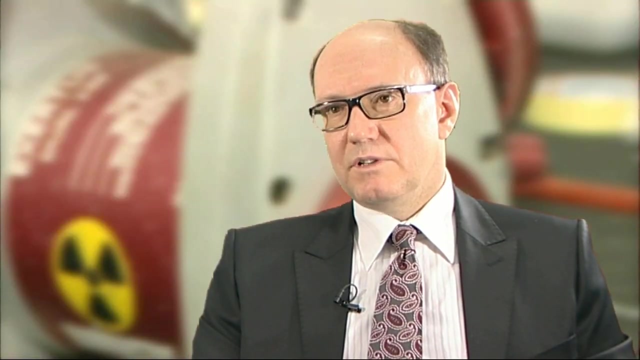 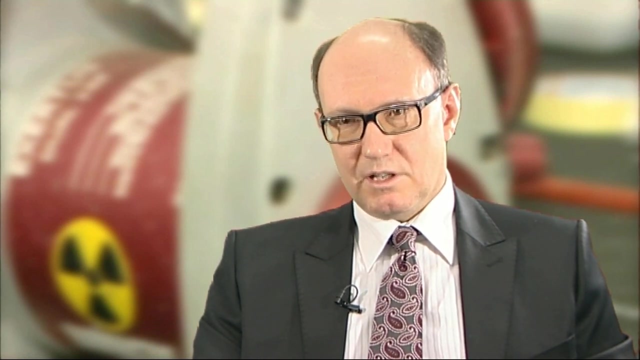 guidelines in the member states. The programme is very wide ranging and covers radiation assessment, monitoring, protection, training, regional workshops and various information services and networks. So the major role of the IEA is to bring the contemporary scientific knowledge to the regulatory language, to the applicable language in legislations, and advocate the 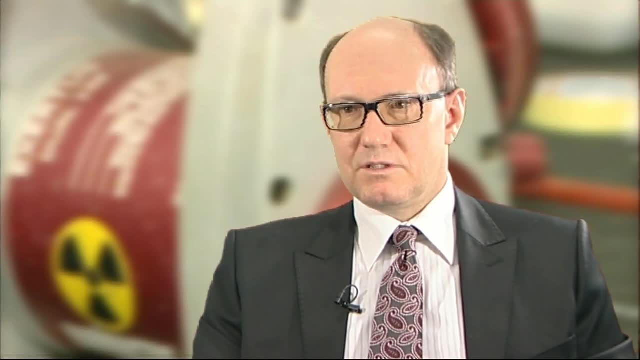 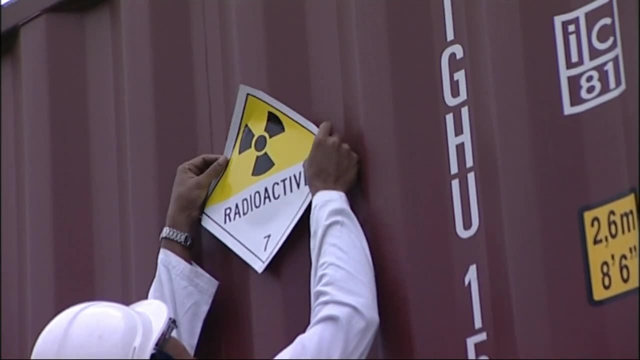 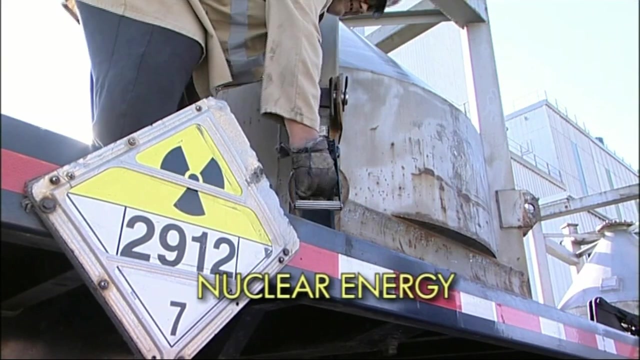 use of these standards in the member states' legislations. The programme concerns itself with all those people around the world whose jobs involve persistent, sometimes daily, potential exposure to radiation. The nuclear energy industry, it seems, is one of them. But it is also one of those industries where radiation itself goes without saying. but 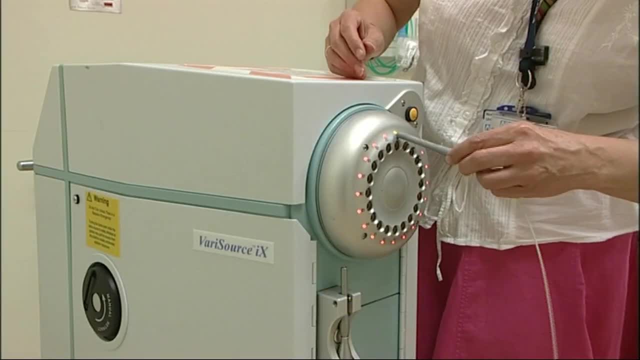 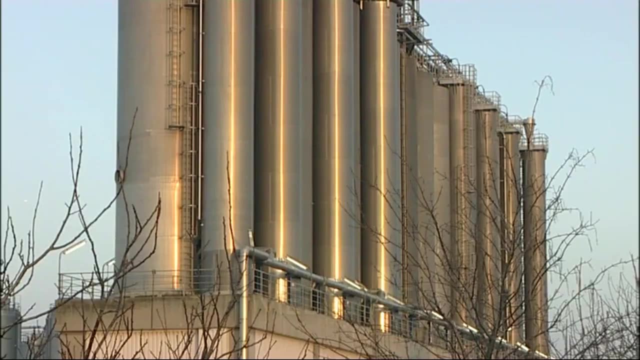 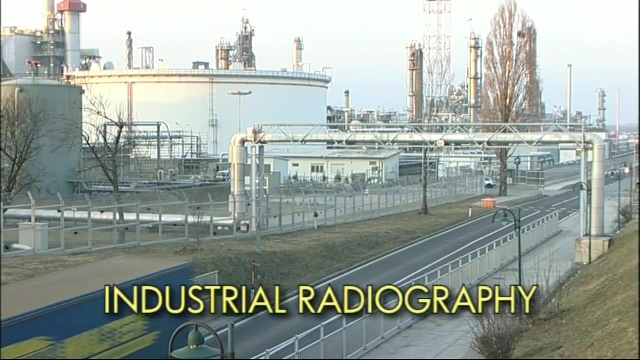 other areas of concern are less obvious, For instance, those working in medical facilities, where radiation is used for diagnostic or therapeutic purposes, Those working in other industries, including oil and gas, where radioactive sources are regularly used, And those working in places that expose them to significant levels of natural radiation. 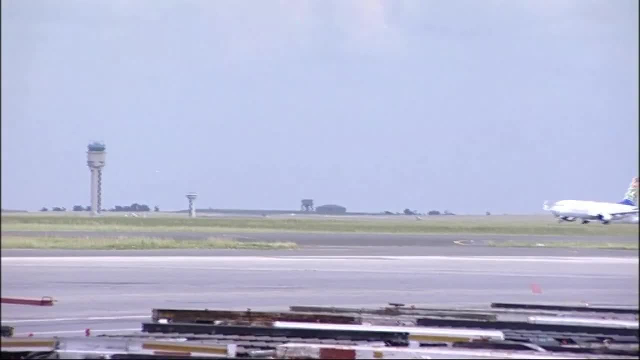 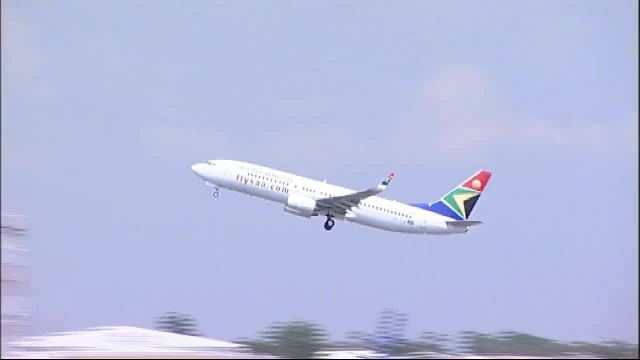 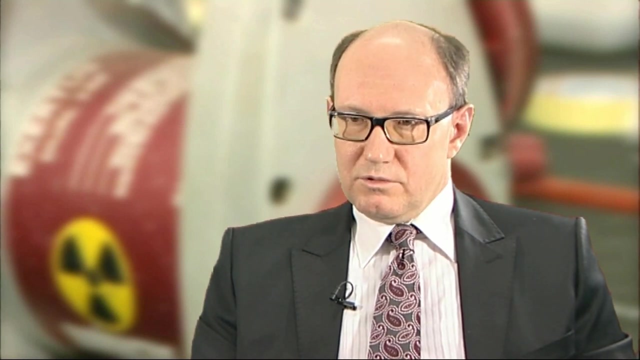 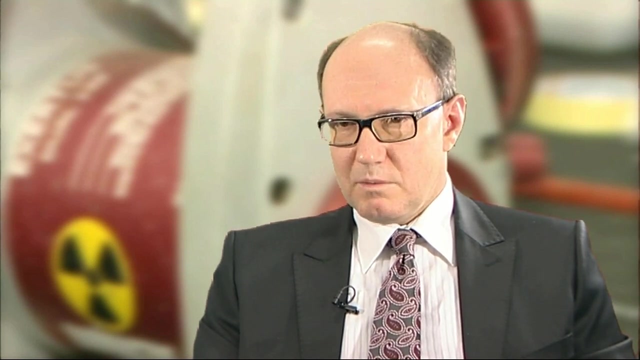 – coal miners, uranium miners and aircrew. The agency is particularly interested in those workplaces where radiation safety regimes are less well established. We have several areas we need to focus on. One is typically nuclear power plants. I do believe the nuclear power plants and the radiation protection programmes are well 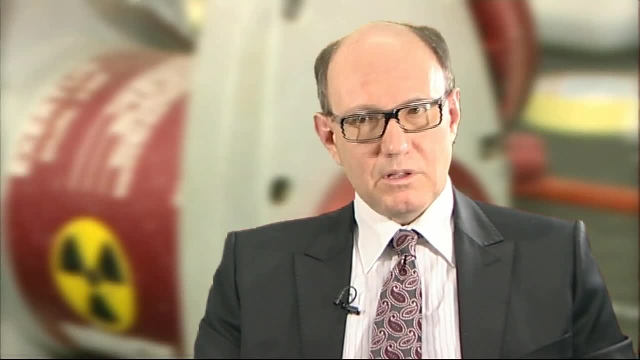 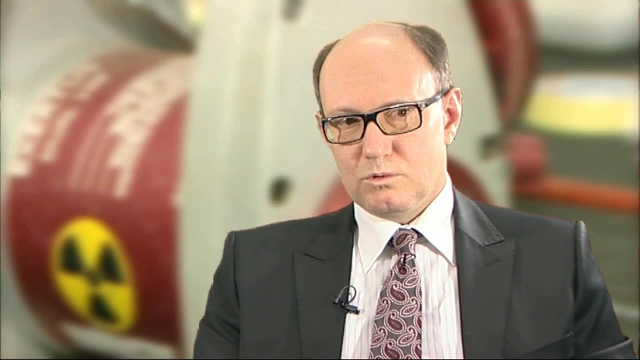 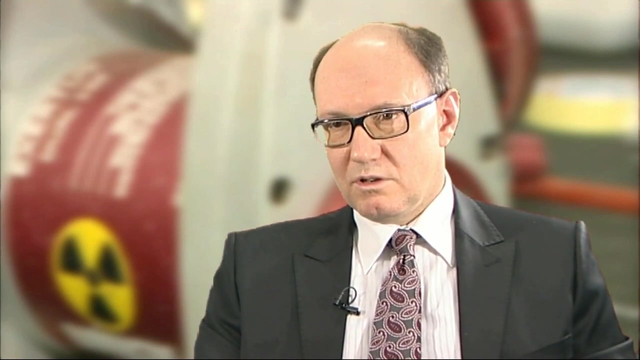 set and well established and observed in most nuclear power plants which we have in the occupational exposure is to direct attention of radiation protection professionals or regulatory authorities in countries to those industries which are not that much under the scrutiny of radiation protection control. This is mining, this is 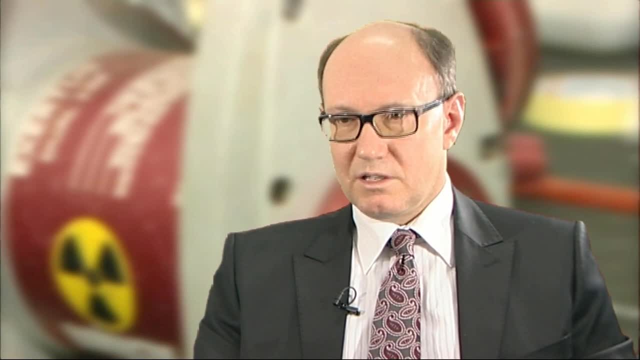 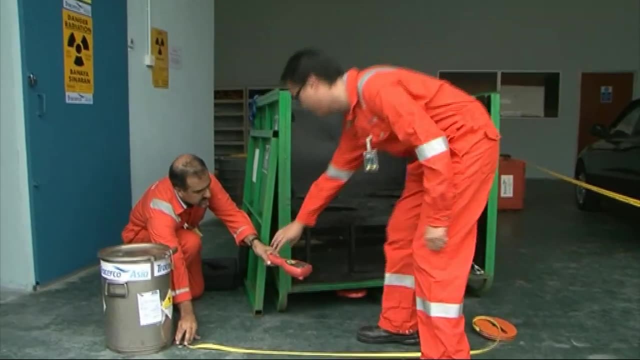 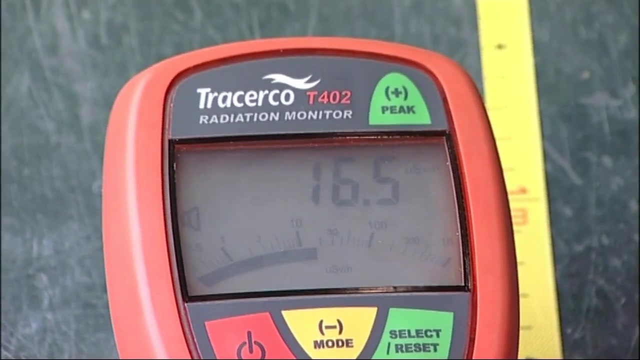 medical field. these are industry, like, for example, industrial radiography, But the principles of radiation protection are the same in all workplaces. They are the consequence of three factors that control the amount or dose of radiation received from a source: The length of time of exposure to the source, the distance from the source and 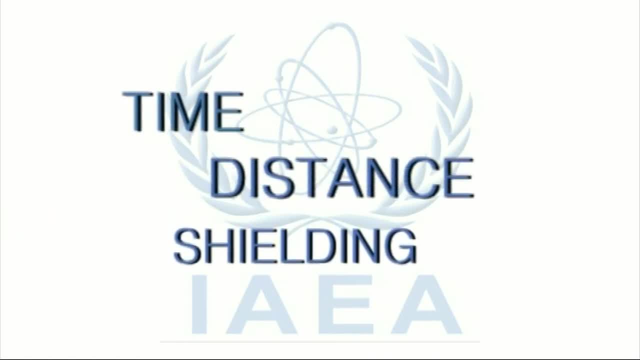 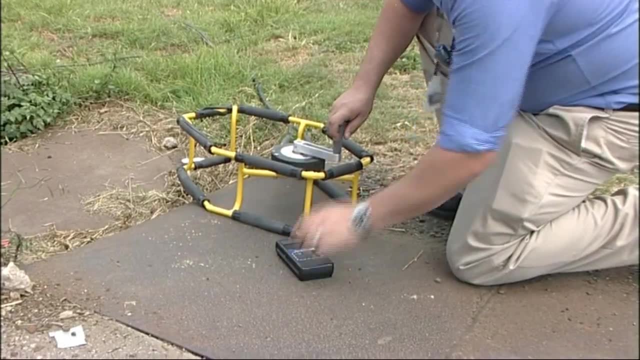 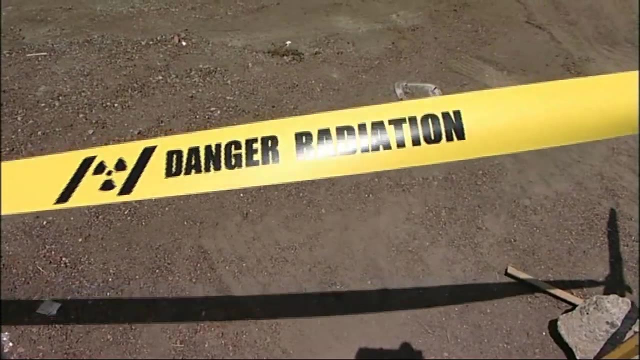 the shielding from the source. Radiation exposure can be managed by a combination of these factors. So the first principle is to limit the time of exposure, Because reducing the time reduces the effective dose proportionately. The second principle is to maximise the distance from a source, Because this reduces the dose. 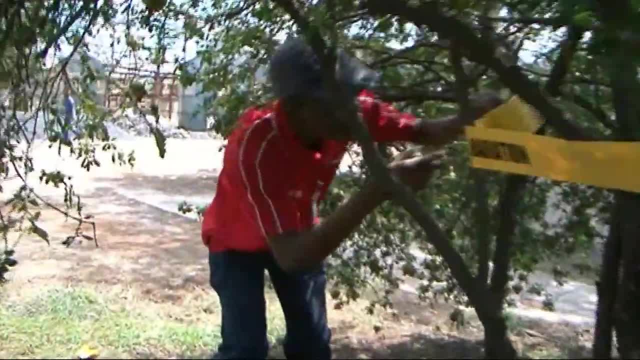 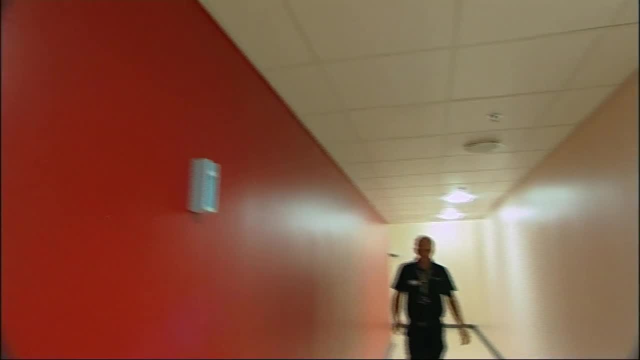 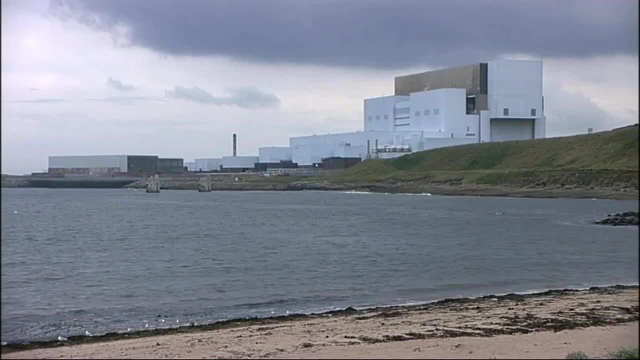 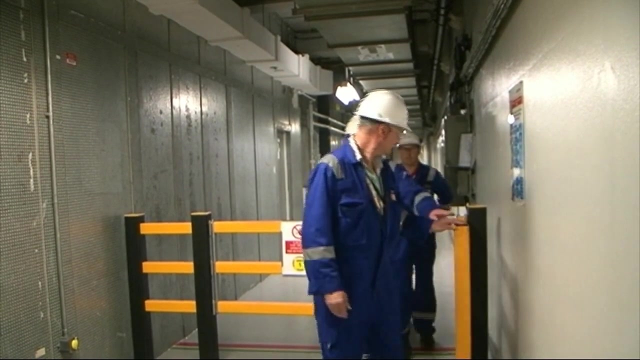 due to the inverse square law. And the third principle is to use shielding to limit exposure, introducing a barrier between the worker and the source. These principles are very well established in the nuclear energy industry, a sector which employs around 800,000 people worldwide, For example here at Tornes in the United Kingdom. 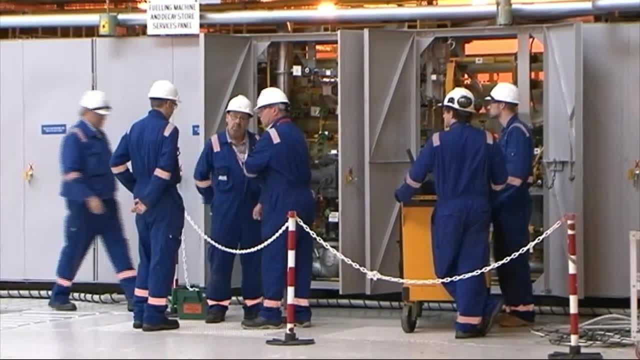 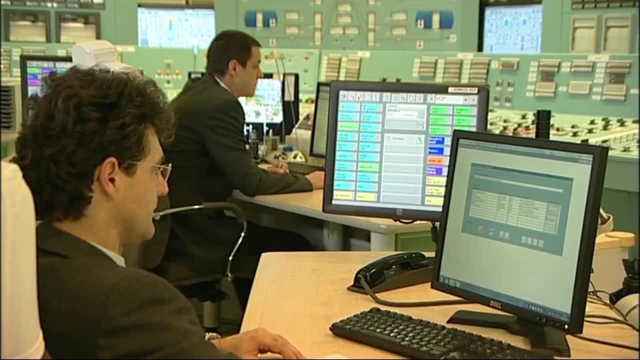 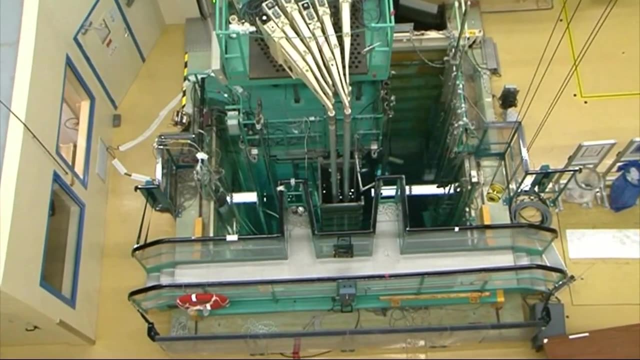 the time that the workforce is allowed to spend here at the top of the reactor vessel is strictly controlled. Similarly, here at the Pax reactor in Hungary, the control room is located as far away from the reactor vessel as possible, And at this small research reactor in Saclay, France, water 7 metres deep acts as a shield. 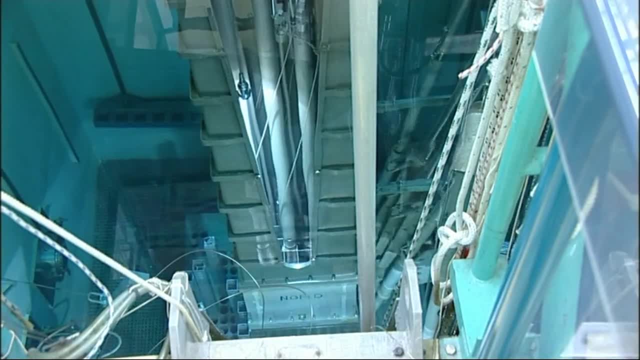 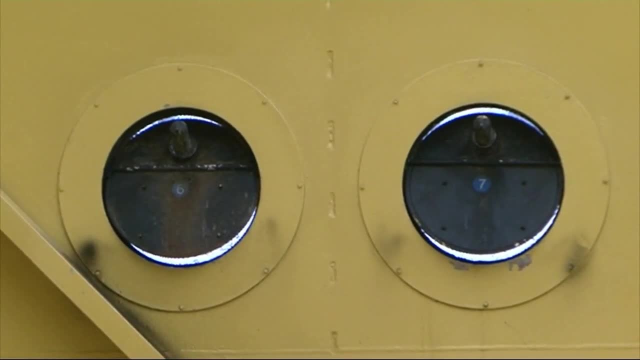 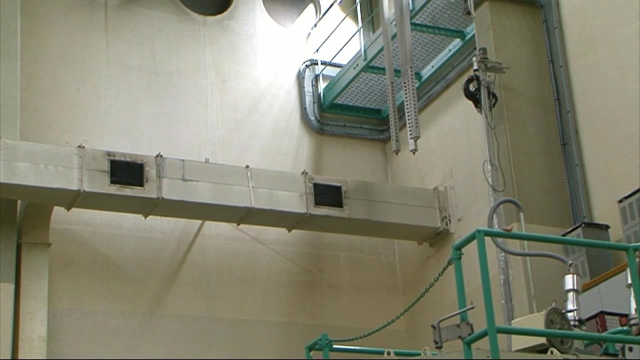 between the core and the reactor hall And at Saclay. as is commonplace with reactors worldwide, the atmospheric pressure in the reactor hall is kept below that of the external environment so as to contain radioactive contamination within the building. These three principles are also to be seen as a very important part of the nuclear energy. 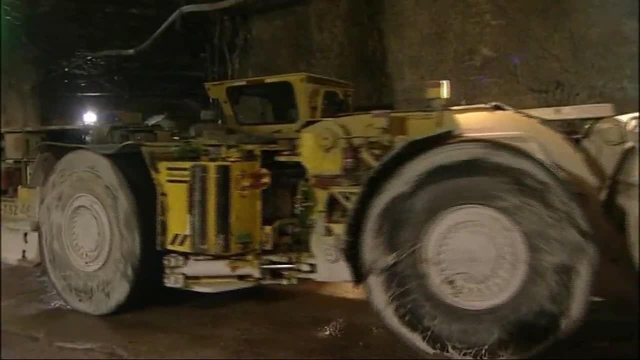 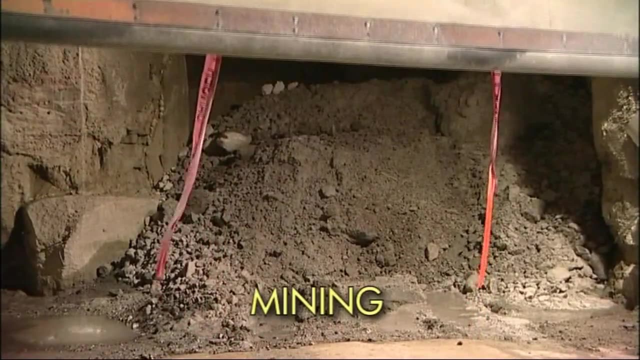 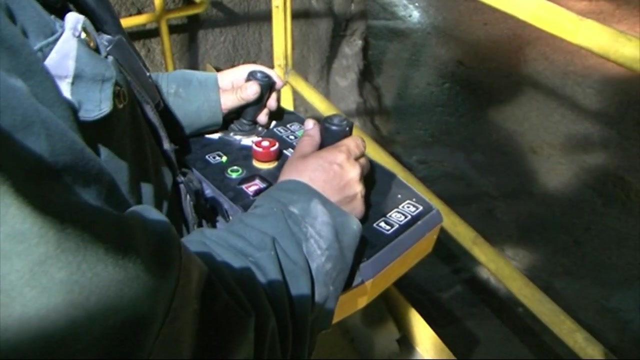 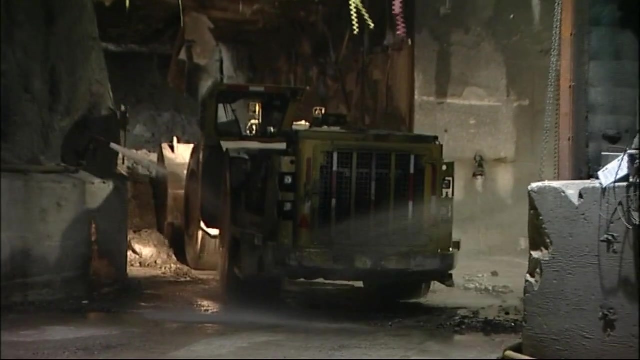 Also to be seen in practice in another important aspect of the Agency's Radiation Protection Programme for the mining industry. Here an excavator is operated by remote control to ensure a safe distance exists between the worker and the radioactive source, in this case uranium ore. 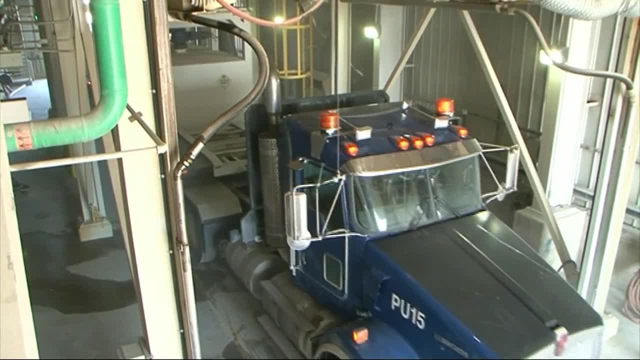 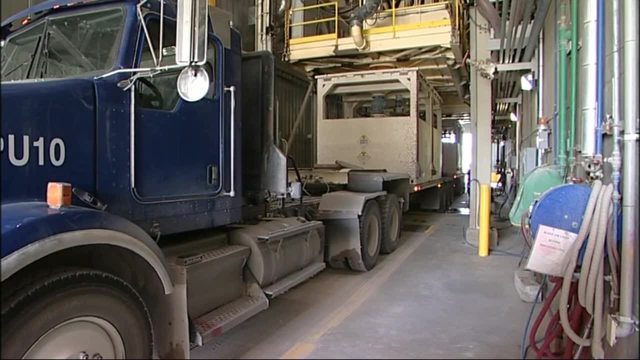 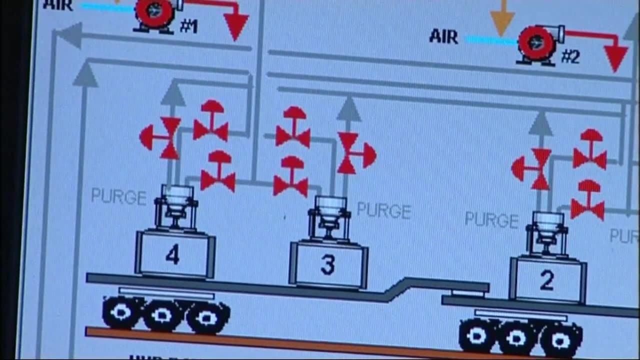 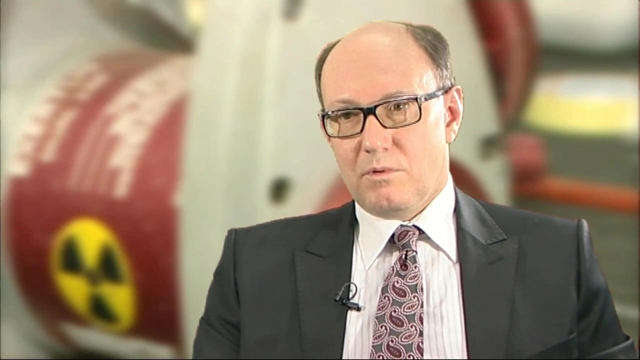 Similarly, at the processing plant the uranium slurry is remotely unloaded. IDEA seat and industrial facility India is also addressing other mining than uranium mining, like coal mining, Emanation of radioactive materials, for example radon, from the minerals without proper ventilation. 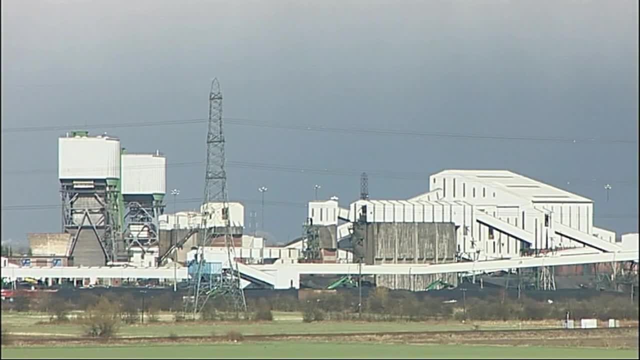 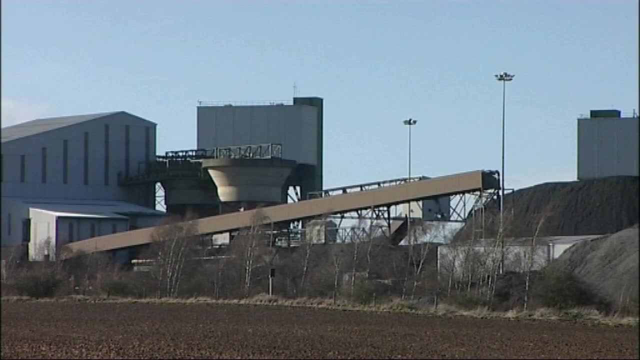 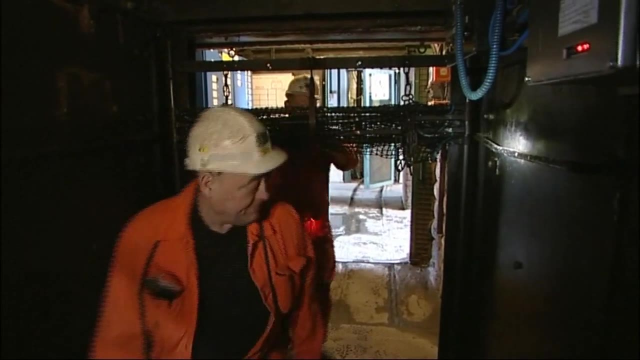 may reach the energy capacity and therefore that is restricted at higher levels. Worldwide, mining for coal is a vast industry. Millions of miners are regularly monitored for exposure to radon. It's a colourless, odourless gas which can be found throughout the world. 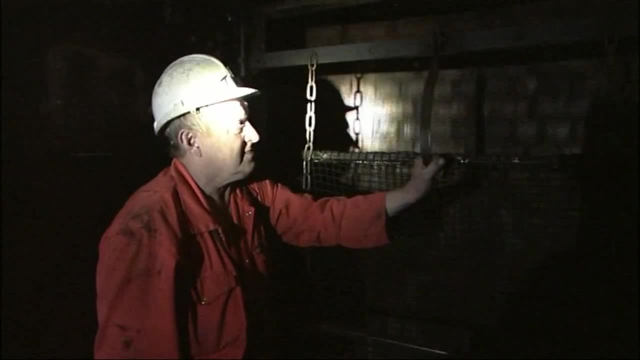 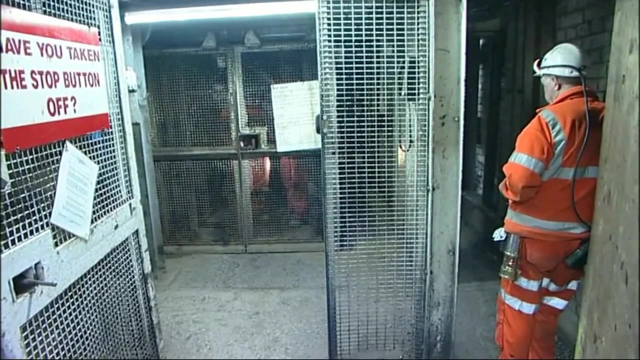 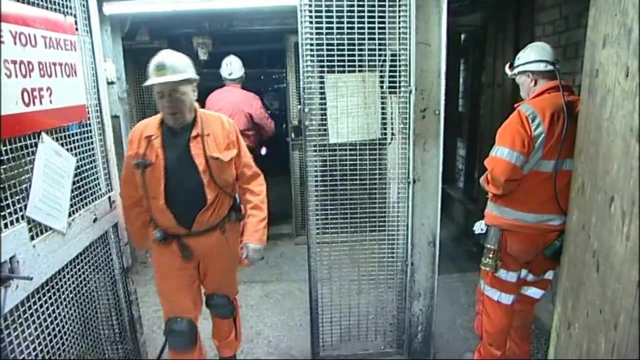 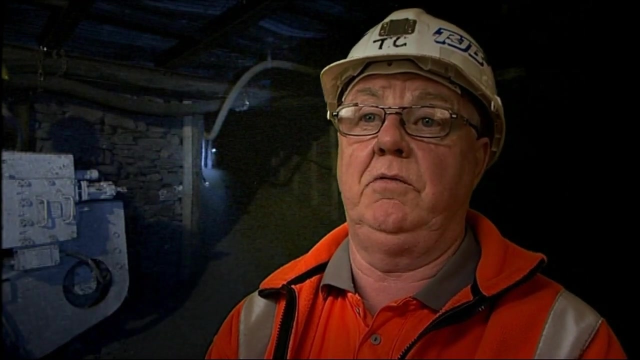 The World Health Organisation has attributed radon gas to being a significant cause of lung cancer, Generally in coal mines. obviously we're always monitoring for gases such as methane. For radon there is two basic methods that we use. We can either use like a small plastic cap which is left in situ in place for a set period. 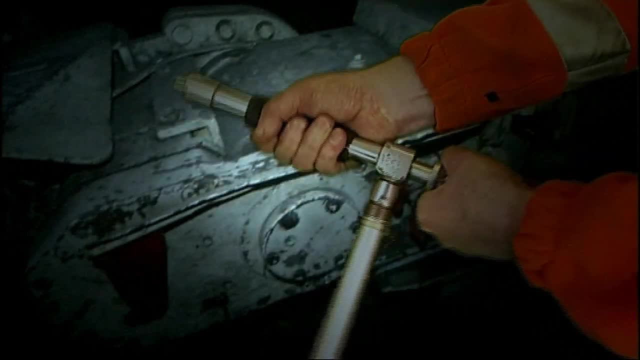 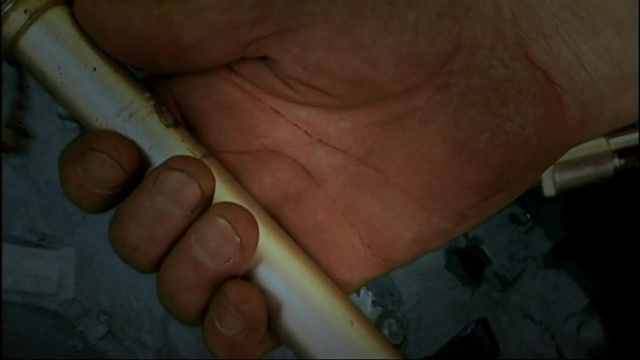 of time. The other method that we generally use is a regression pump. It looks a little bit like a bicycle pump. We will then take an air sample in designated parts of the mine into that pump itself. It's retained within that pump. It's in the tube. 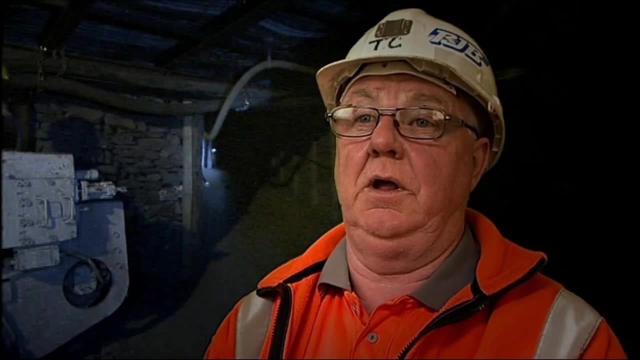 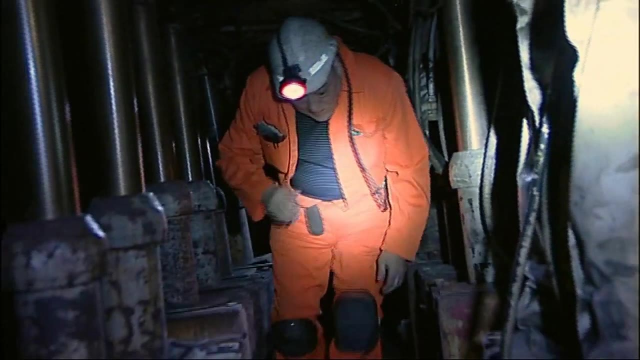 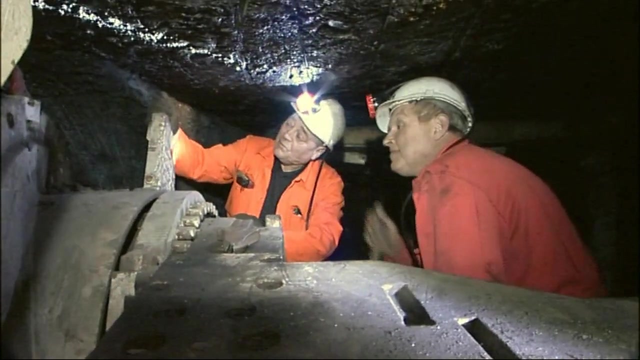 It's sent away for analysis. If we discover that we have radon gas in the mines of any levels above 400 becquerels per metre cubed, then obviously we need to then go into what we call an action level. Now we'll start by completing the risk assessment. 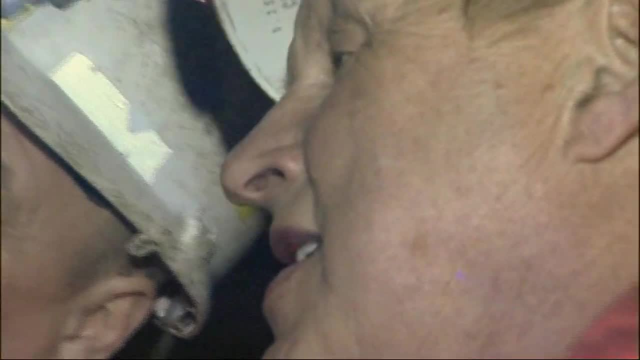 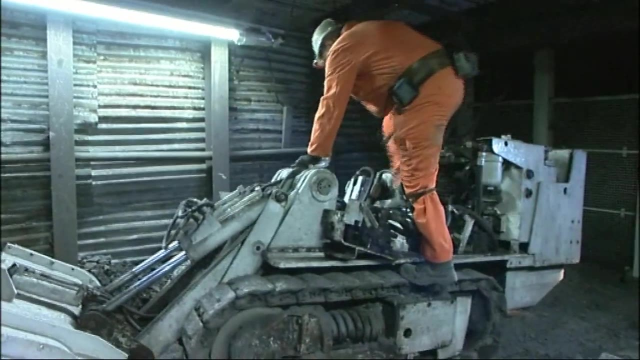 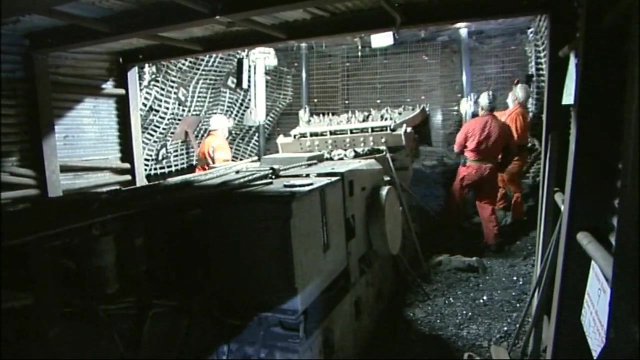 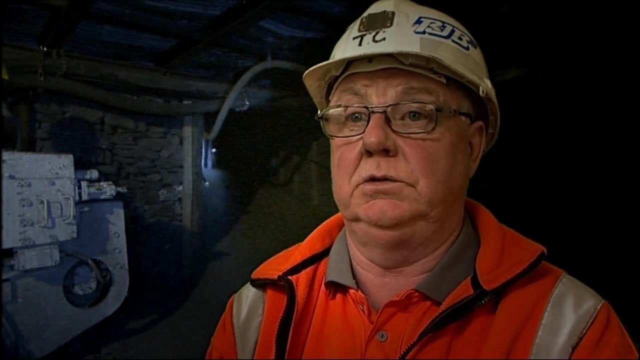 It may be asking us to restrict the hours that some of the mines are actually working underground so that their exposure levels are reduced. We also need to increase the amount of medical surveillance that we do. We have a number of health and safety rules, regulations and acts which are already in. 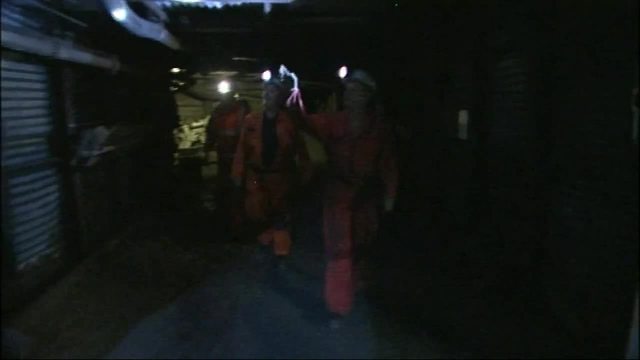 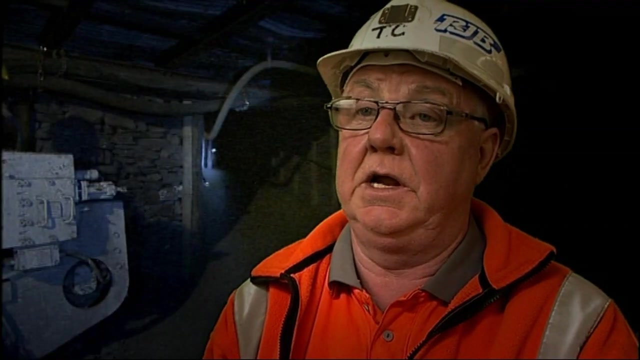 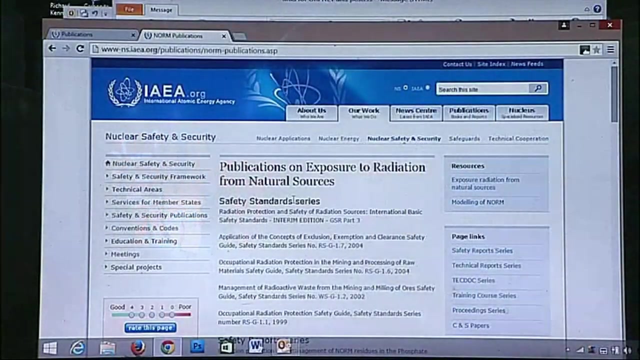 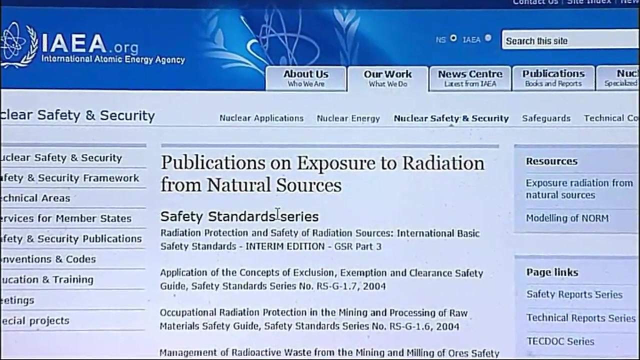 place in the UK mines. However, we do receive a number of directives from the European Union. The European Union receive their advice and guidance from the International Atomic Energy Agency. The International Atomic Energy Agency has a dedicated programme on naturally occurring radioactive materials, NORM. 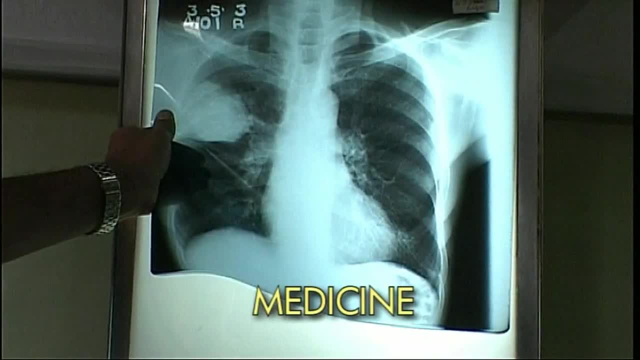 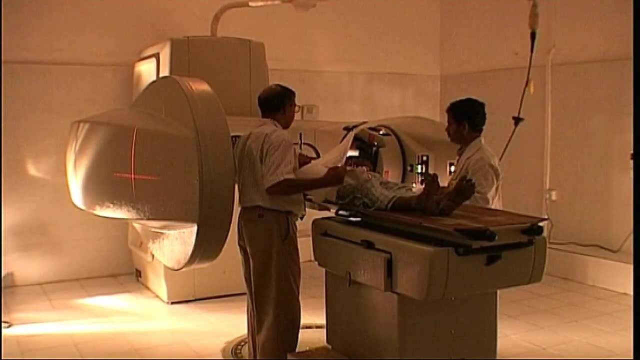 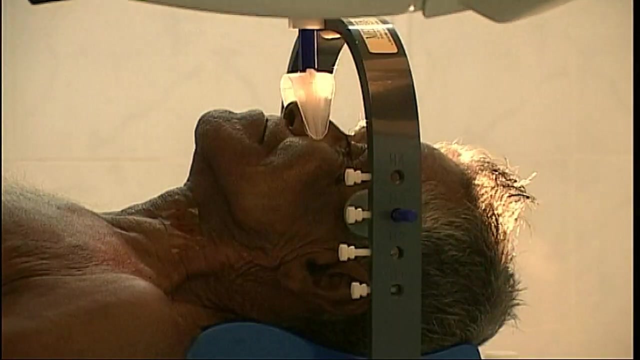 Another important area for the Agency's radiation protection programme is in medicine. Ionising radiation is used very extensively both for diagnostic and therapeutic purposes, And safe working practices include the use of radioactive materials. in the use of radioactive materials, These materials are essential both to protect the patients themselves and the workforce. 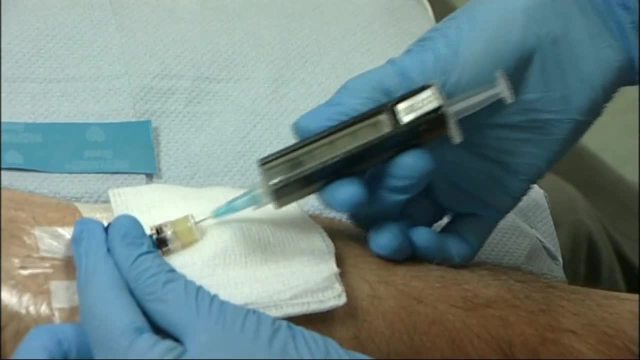 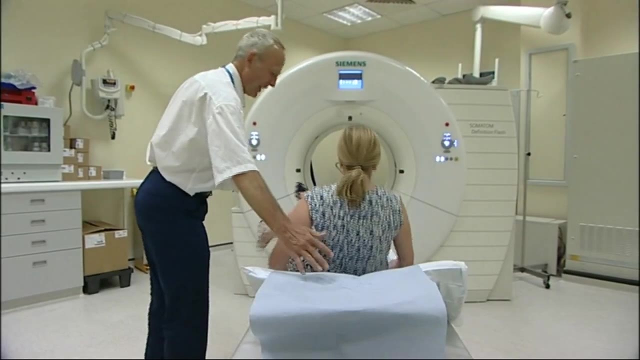 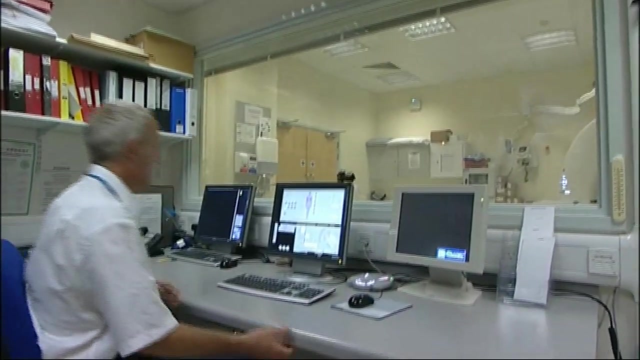 In this unit in a hospital in the United Kingdom, the nurse is protected from the radioactive tracer by using a lead-lined syringe. Similarly, the operators of this PET scanner withdraw through lead-lined doors to a control room behind a leaded glass window when the scanner is in use. 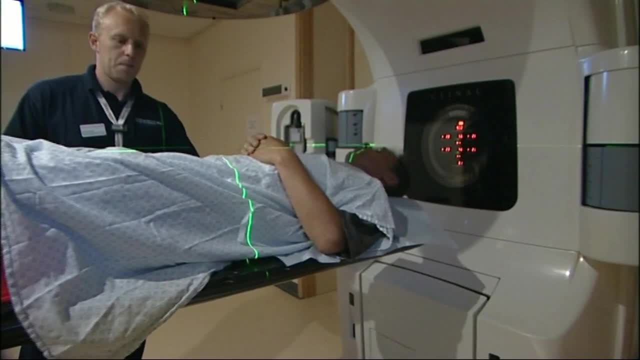 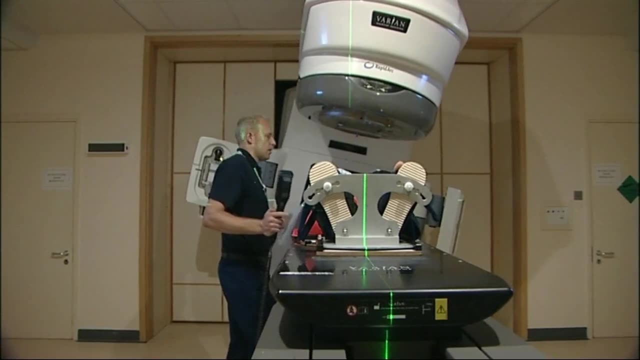 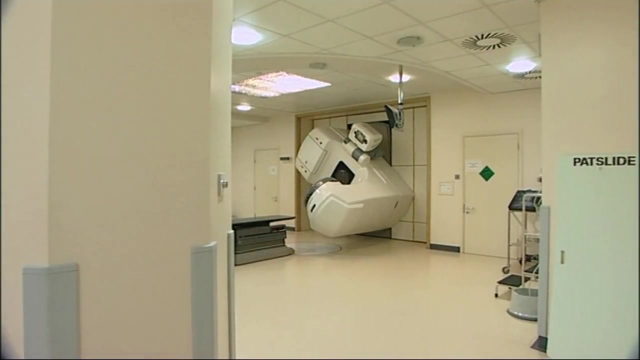 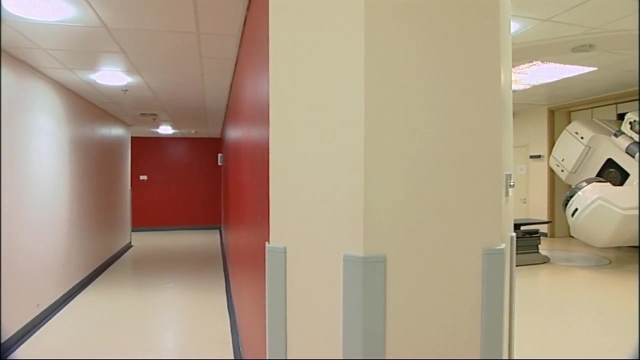 The radiation doses used in therapeutic medicine, particularly for the treatment of cancer, are much higher At this hospital. thinking about radiation protection began with the design of the building. Note the thickness of the walls and the way in which the design of the corridor prevents. 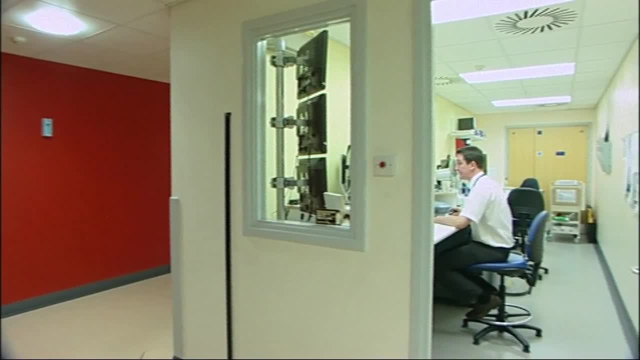 high energy beams of radiation. This is the first time radiation protection has been done in a hospital in the United Kingdom, And in all units in the hospital constant monitoring is used to avoid contamination. Here, a treatment room is being checked for traces of radioactivity. 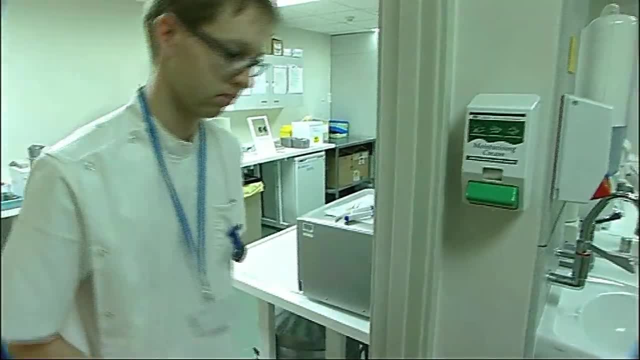 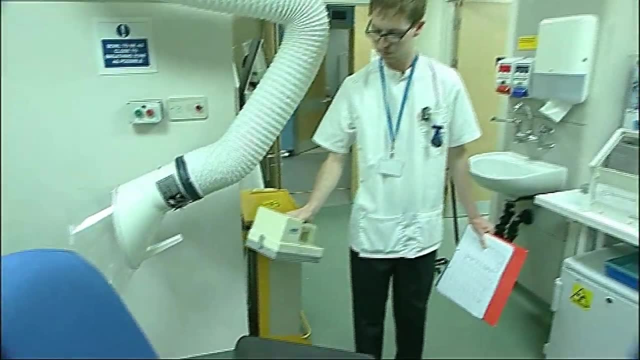 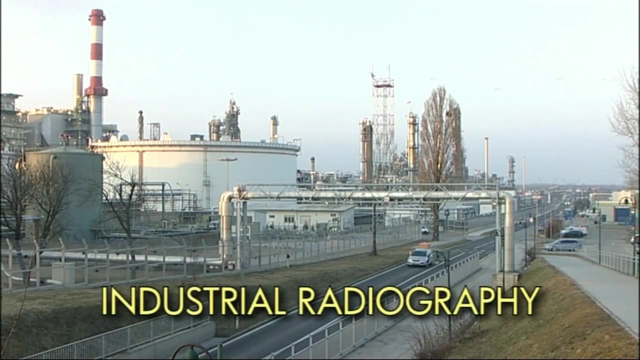 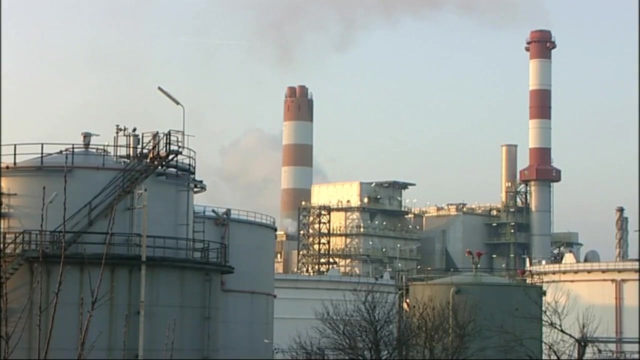 Additional tests are also being done in the hospital for radiation protection. Ionising radiation is used extensively in the testing and grading of radiation coating. The main area of particular interest in the IAEA is industrial radiography. Ionising radiation is used extensively in the testing and grading of radiation, which 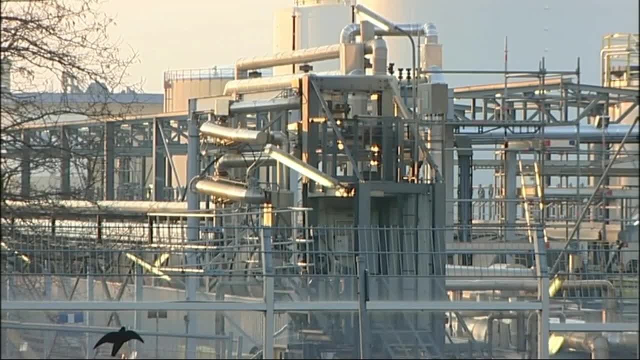 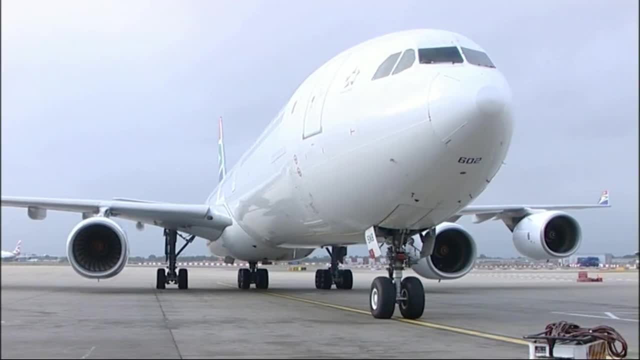 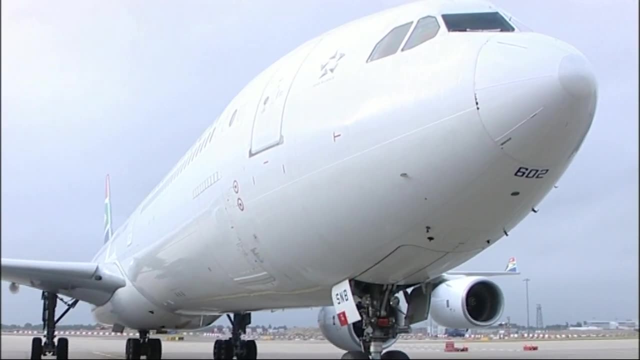 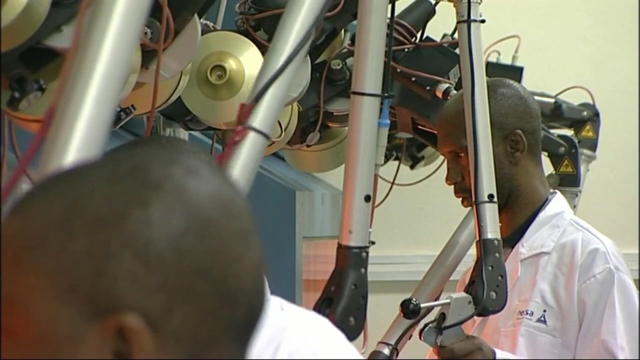 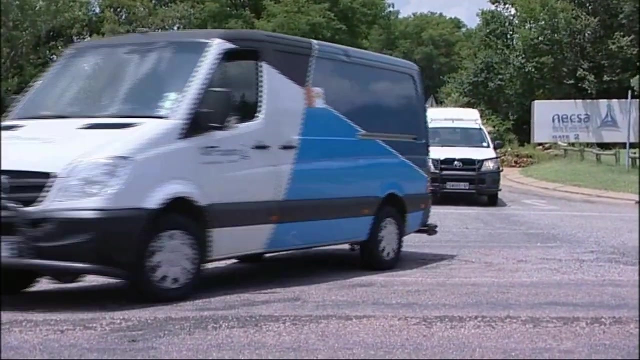 and grading of wells on pressurized piping pressure vessels, high-capacity storage containers, pipelines and some structural wells, including those on aircraft wings. The radioactive sources used for this purpose include iridium-192, selenium-75 and cobalt-60.. Here outside Johannesburg, NTP Radioisotopes is manufacturing. 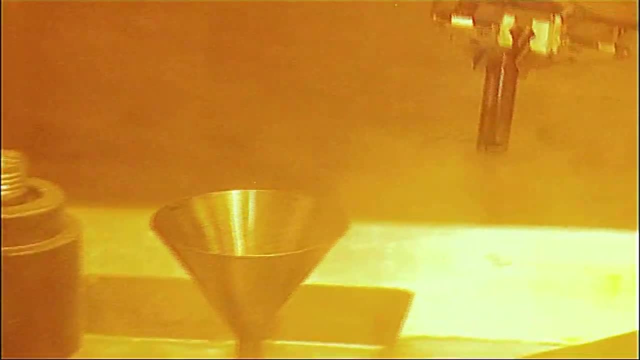 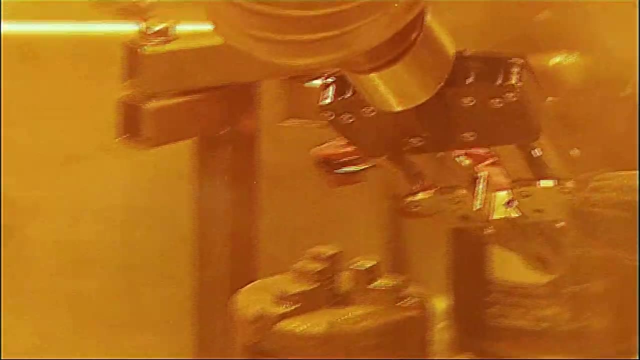 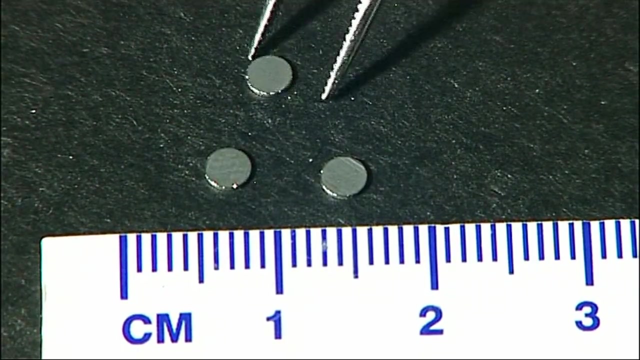 iridium in a research reactor and then packaging it into a form usable as a source for industrial radiography. These iridium-192 sources are minute, measuring three millimeters in diameter and only 0.3 of a millimeter in thickness. 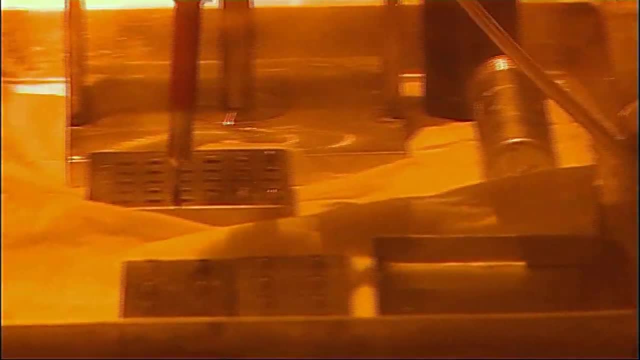 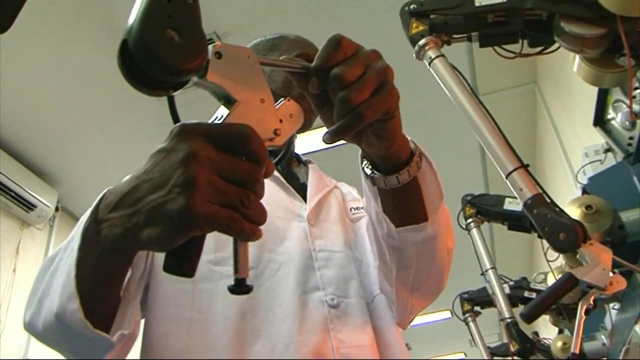 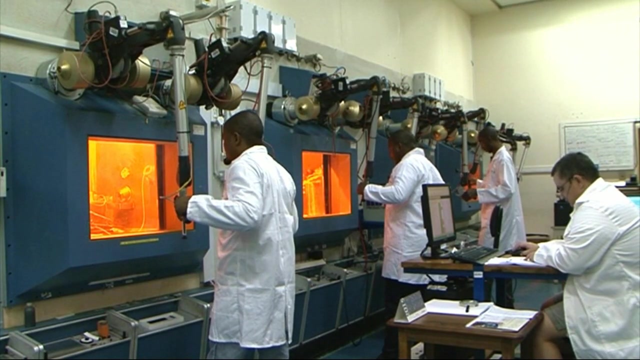 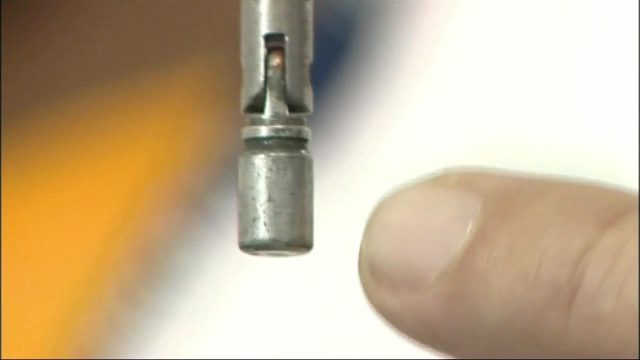 But they're a powerful source of gamma radiation which can penetrate a hundred millimeters of steel. The hot cell operators are protected by 250 millimeters of lead shielding around the sides of the cell and leaded glass at the front, which is nearly a meter thick. The tiny sources are loaded into. 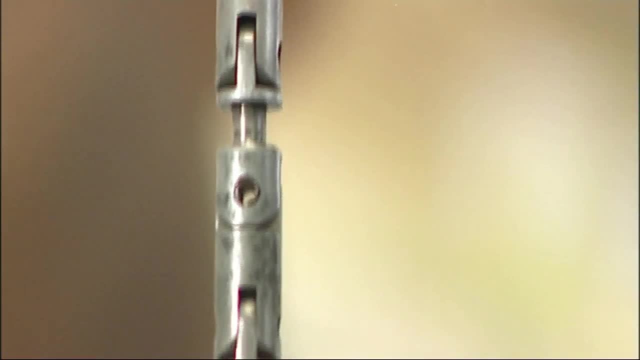 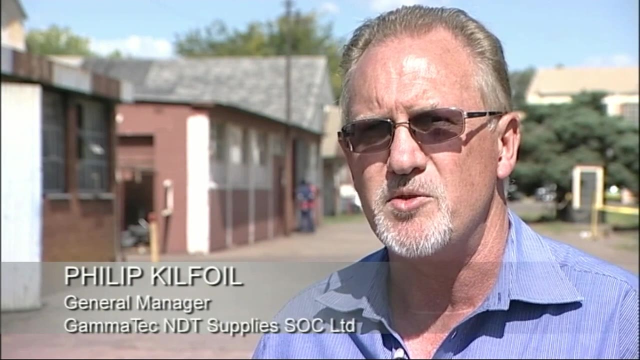 capsules, which are then connected to a jointed cable called a pig's tail. Radiation is like light: it travels in straight lines. so it's very important that, when the source is housed within the projector, that no radiation escapes the front or the back ports of the projector. To this end, the source 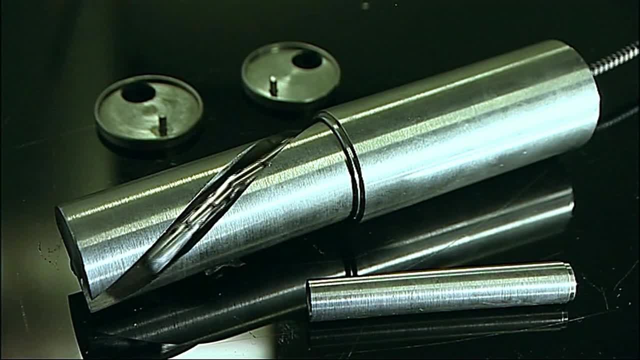 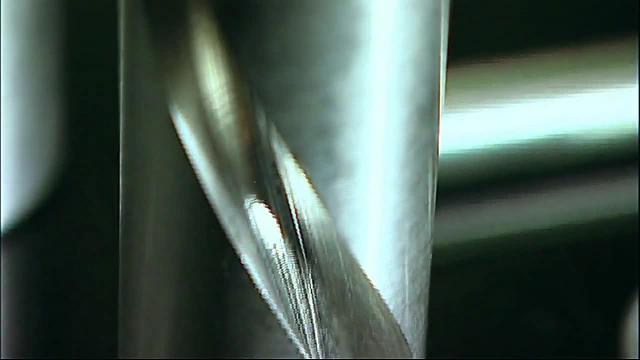 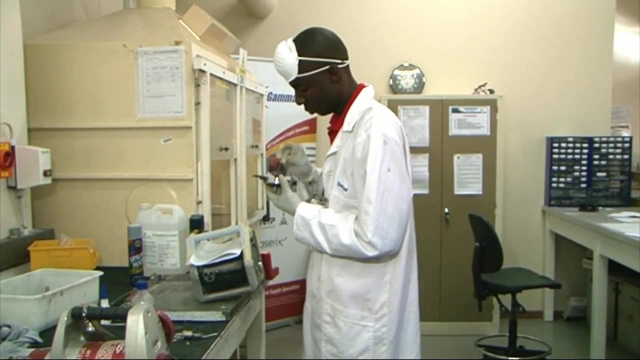 assembly is designed of tungsten links which prevent radiation from leaking out the back of the projector, and there is a tungsten labyrinth which is in the form of a spiral that prevents radiation leaking out the front of the projector. In a workshop at NTP site near Johannesburg, the ship's 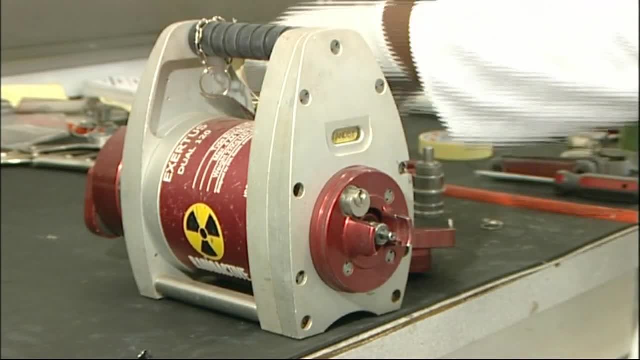 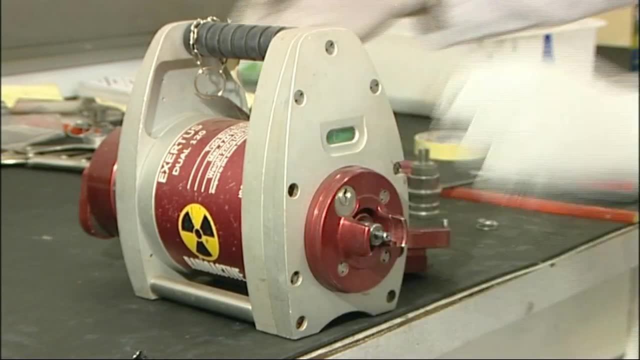 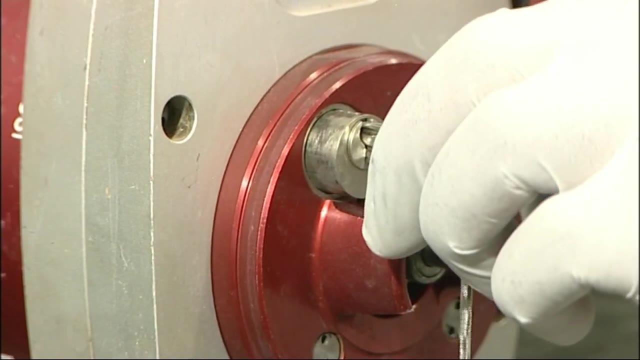 shielded projectors used to house the capsules containing the radioactive source are checked and serviced every time they're loaded with a new source. In addition to the labyrinth, the projectors are designed with a key operated interlock system to prevent inadvertent removal of the source. 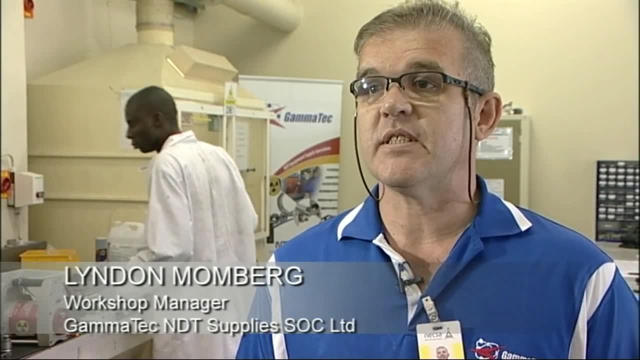 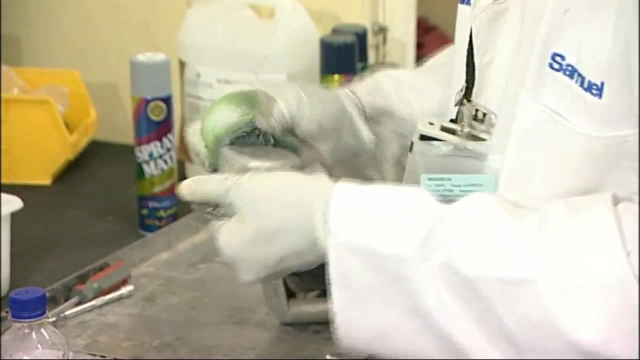 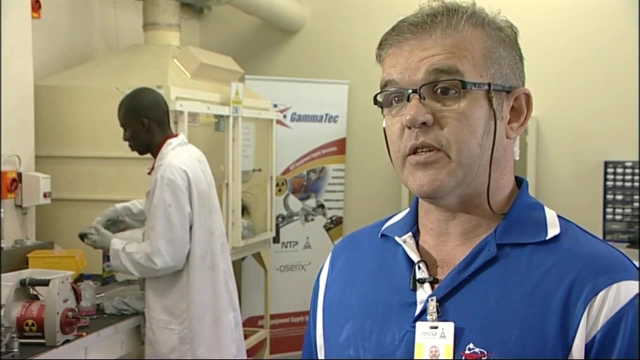 Gamma Tech's approach to safety is three words: safety, safety, safety, Always safety. At the moment, our technician is busy cleaning a duel. This is part of the service, of every single service. Locking mechanisms will be checked. we'll ensure that couplings fit correctly, that the lock 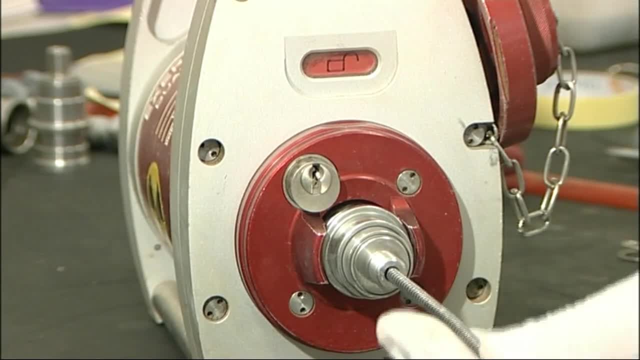 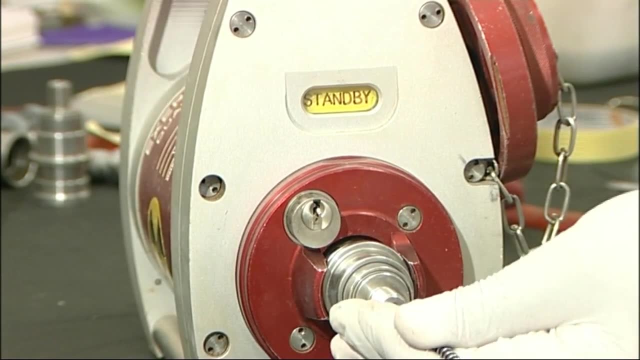 moves freely, and we'll use a dummy pigtail to make sure that the movement of the pigtail in the projector is safe and that the lock engages every time. At the rear of the hot cells is the so-called red area, where the sources in their 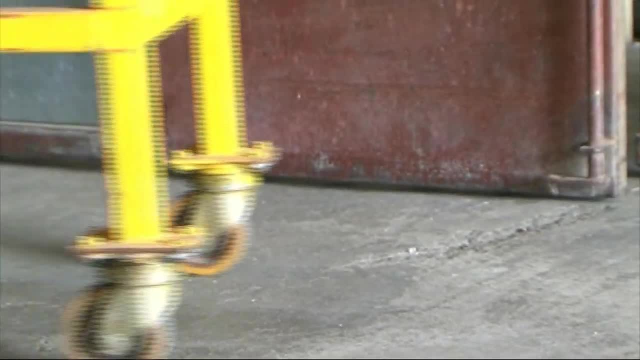 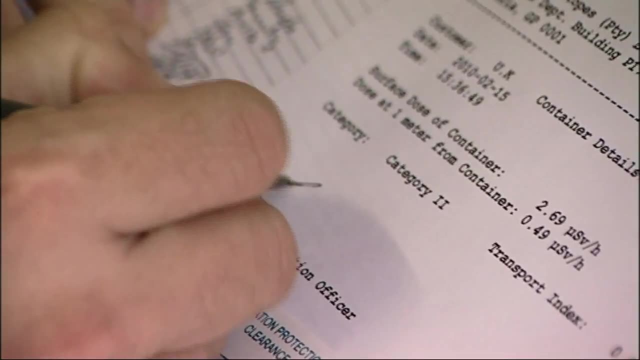 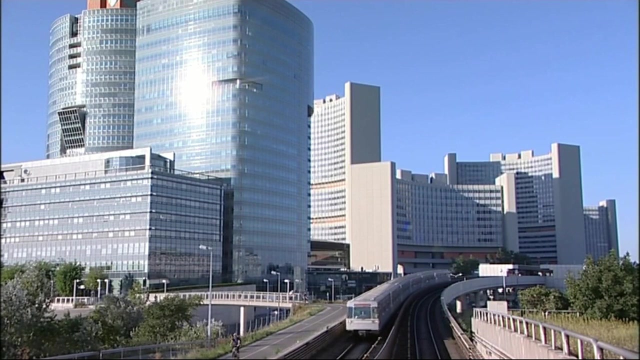 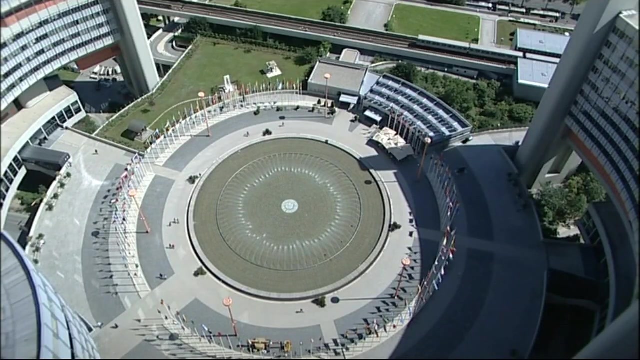 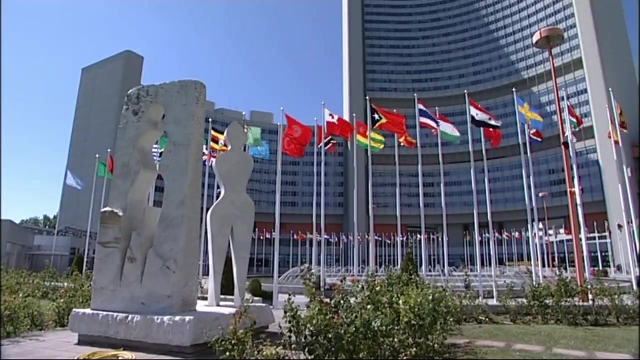 containers are brought out to the dispatch area where they're placarded, checked for radiation- The source is the radiation protection officer. They can now be delivered to the end user. the radiographer- Industrial radiography- does not have a good safety record and is of particular concern. 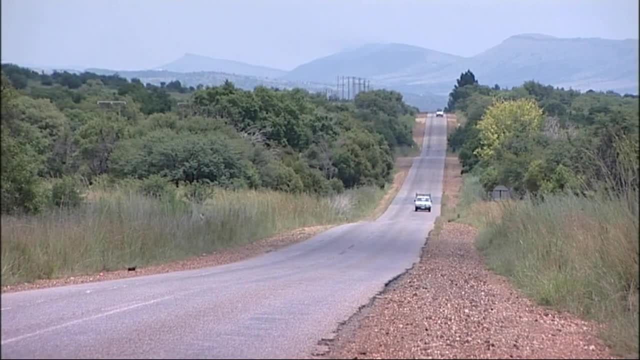 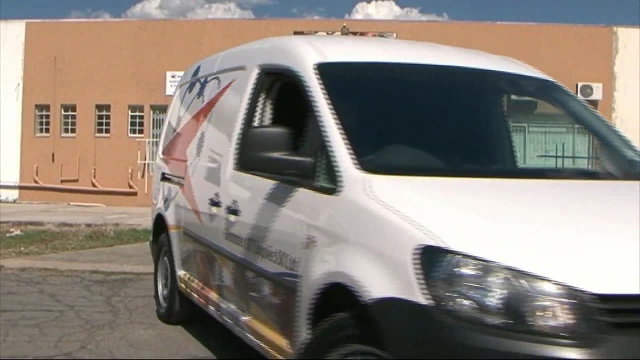 to the IAEA. In some parts of the world there are operators using strong sources in remote sites with little supervision, especially when compared with workers in the nuclear field Here in South Africa. this distributor of radiography projectors values the recommendations and guidelines provided by the IAEA. 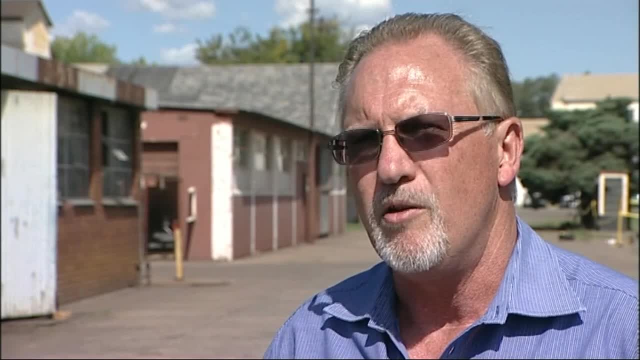 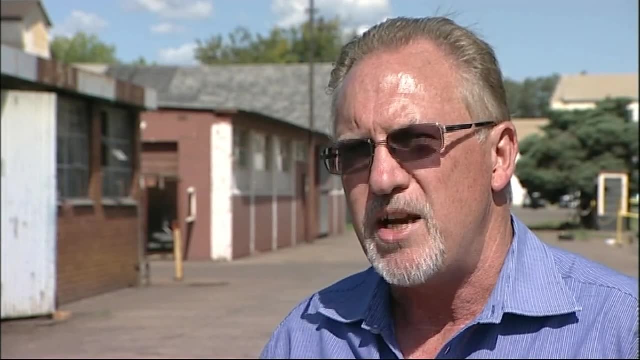 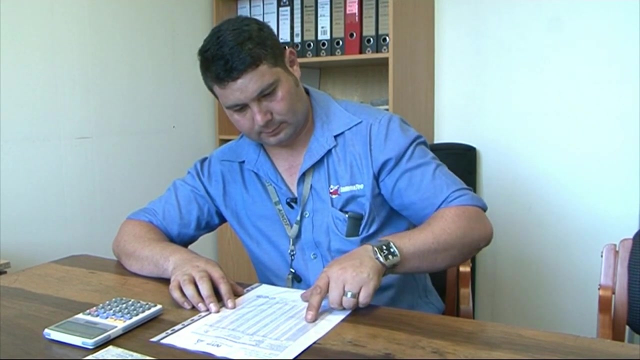 The IAEA rules and regulations form the backbone of the South African Department of Health's rules and regulations for radiography in South Africa, And radiographers are trained in accordance with these rules and regulations Before going out into the field. the radiographer will calculate both the required safe distance. 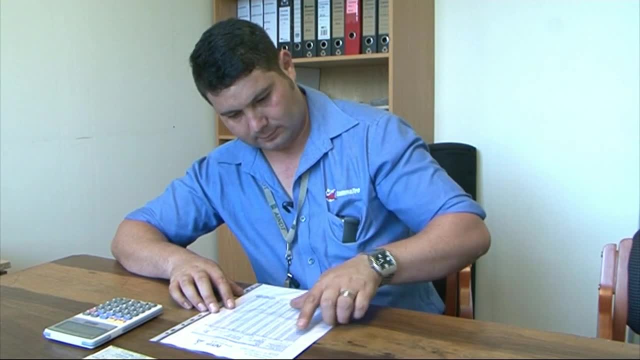 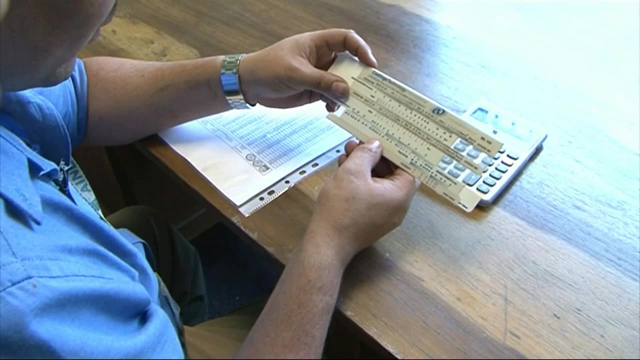 from the source to the safety barrier and the distance from the source to the safety barrier. The priorities are the risk tolerance of radiation and the time necessary for the exposure. For this he'll use an internationally accepted radiation safety principle for minimising radiation doses and releases of radioactive materials. 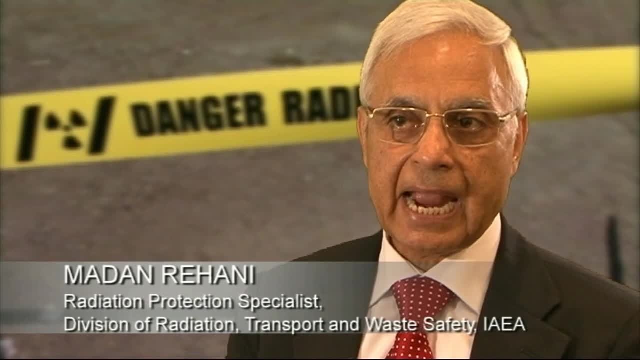 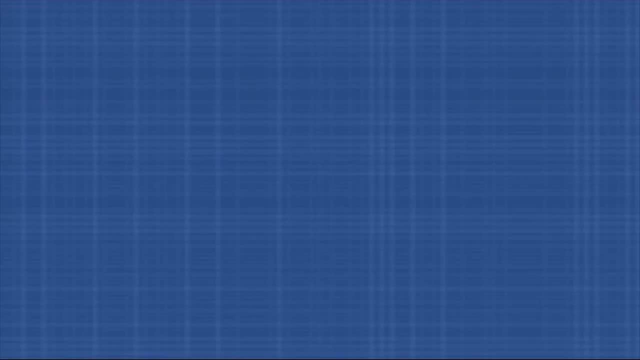 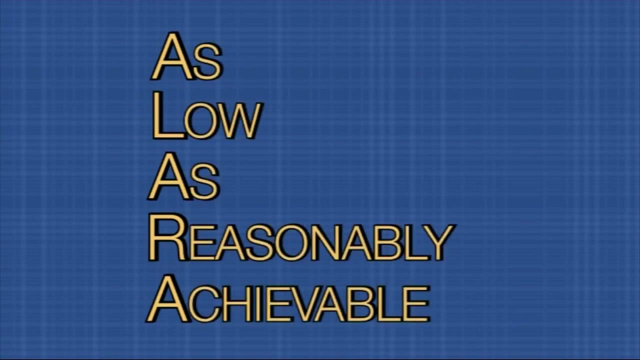 The International Commission on Radiological Protection had developed the concept of As Low as Reasonably Achievable. The acronym is Alara. The International Commission on Radiological Protection has developed the concept of as low as reasonably achievable. The acronym is ALARA. We in radiological professional feel that this is a very important tool. 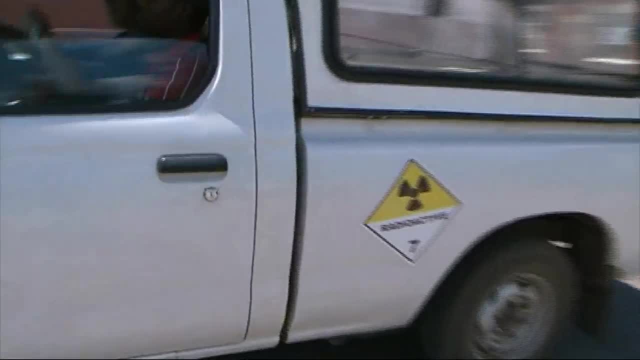 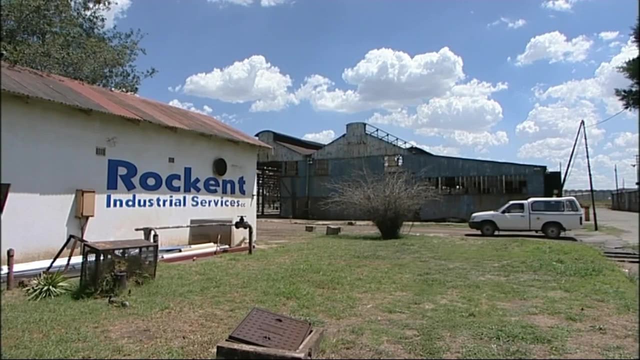 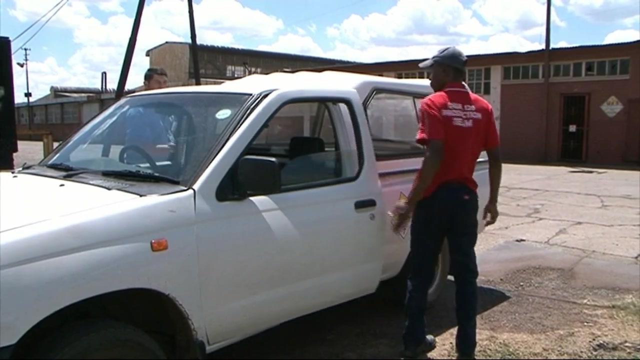 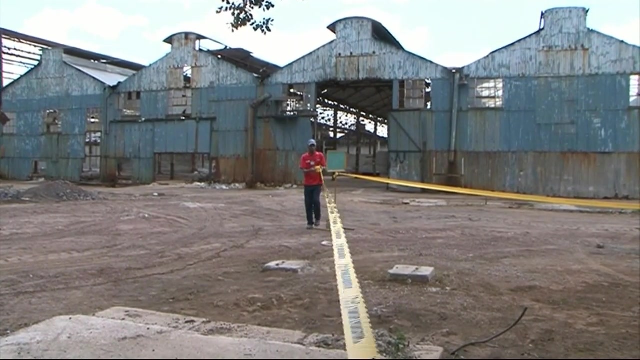 ALARA is not only a sound safety principle, but it is a regulatory requirement for all radiation safety programmes. It's one of the cornerstones of the IAEA's approach to radiation protection. Once on site, the first step is to set up the barrier to keep people at a safe distance from the source. 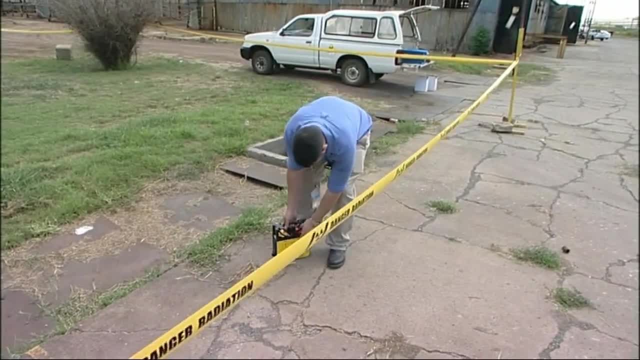 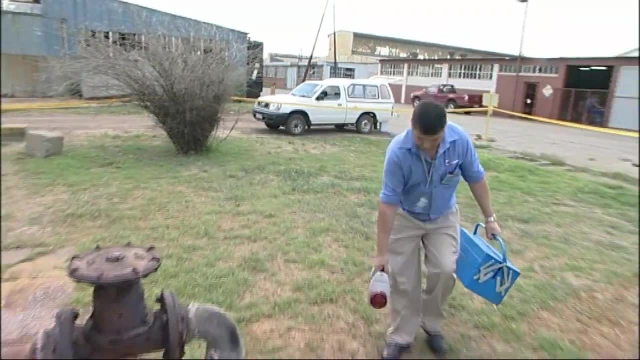 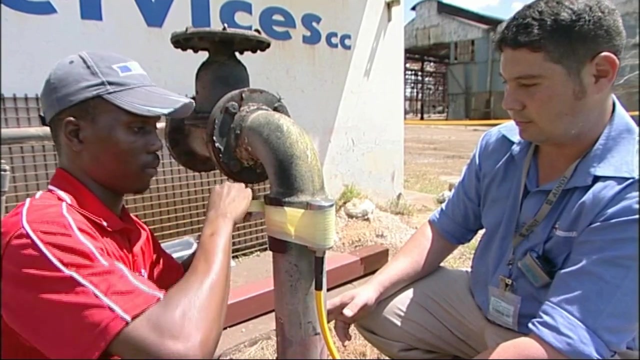 An environmental radiation alarm and a slave are set up at the boundary and checked. The radiographer also has a personal dosimeter. The projector can now be set up. A tungsten collimator with a 60 degree angled port is taped onto the pipe and the film is taped onto the opposite side. 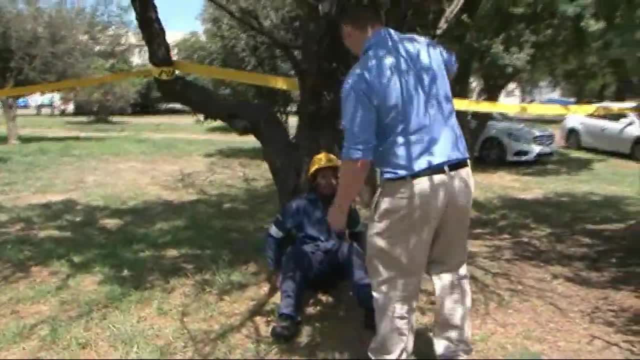 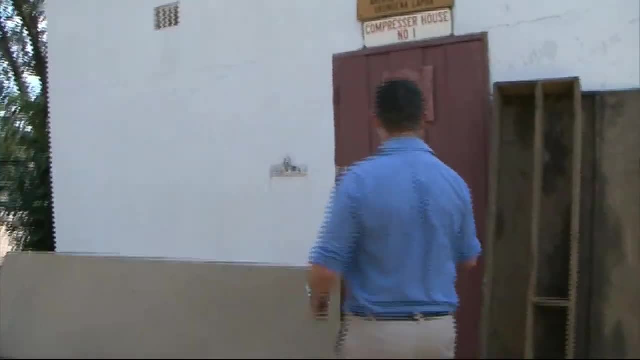 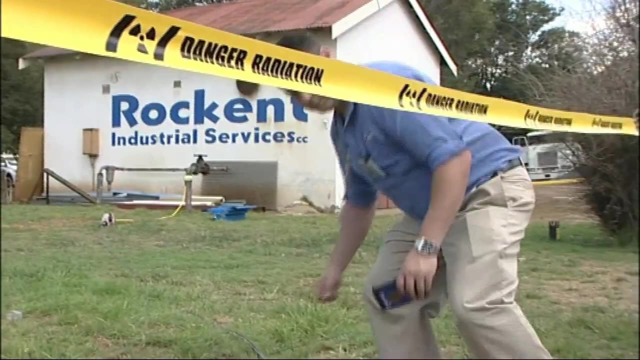 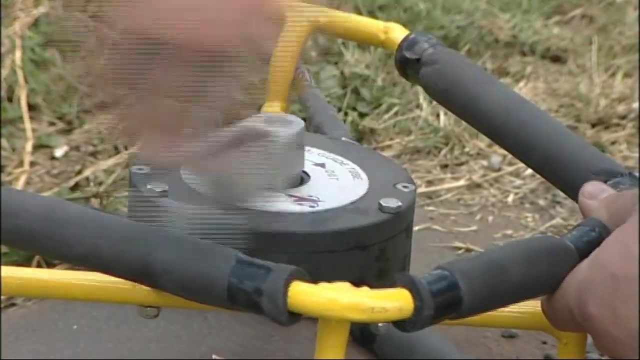 The area is then cleared of people. Just get out the barrier, please. The adjoining properties checked and the perimeter radiation levels checked. The radiographer and his assistants step outside the barrier and the preparations are now complete. The yellow guard is set up, The guide tube allows the source to be wound out of its shielded housing. 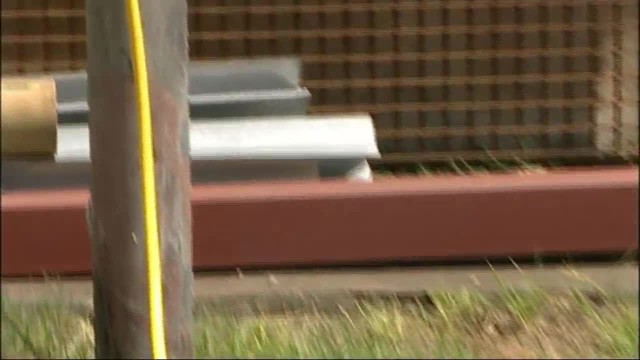 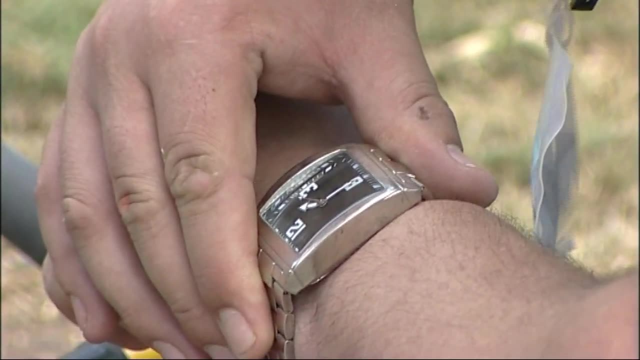 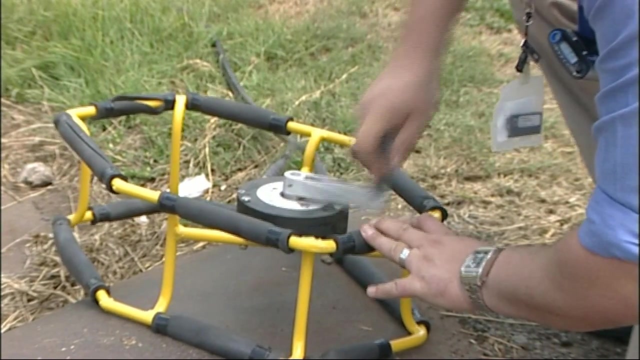 in the labyrinth inside the projector and into the collimator. As soon as the source is out of its shielding in the projector, it sets off the environmental radiation alarm. After timing the exposure calculated in the office, the source is wound back in. 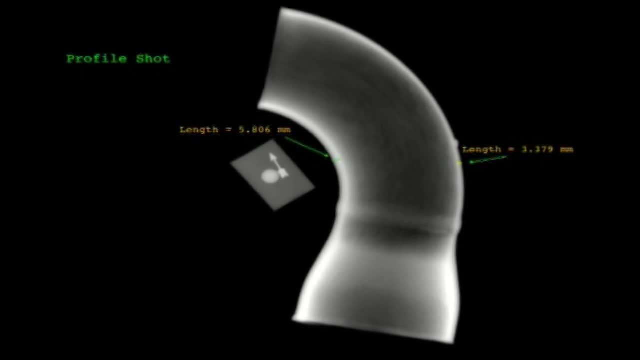 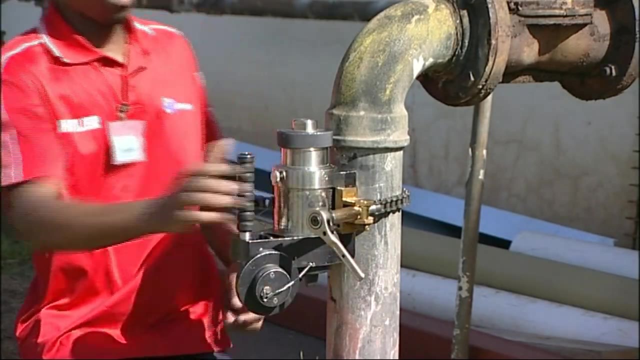 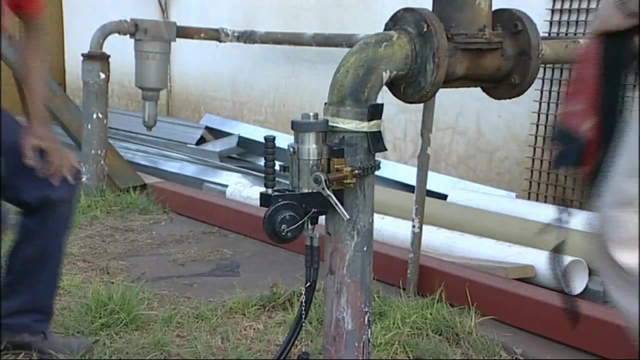 When the film is processed, a detailed examination can be made of the metallurgical integrity of the pipe. A safe and quite new alternative to this method is to use a shielding blanket that limits the spread of the radiation. But whatever the advances in technology, 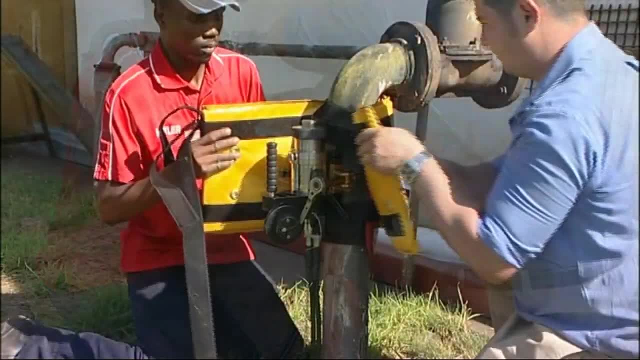 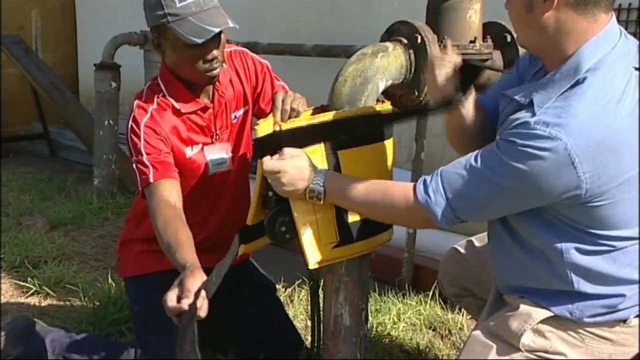 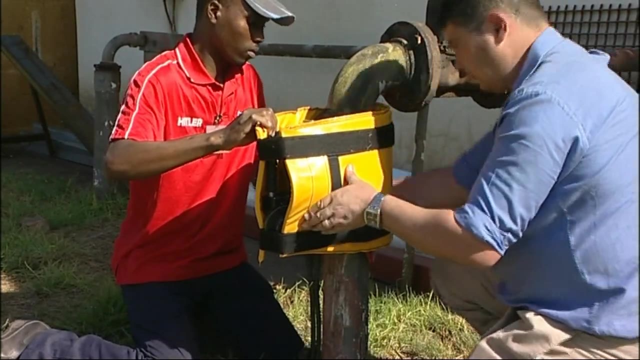 radiation protection is ultimately the responsibility of the individual workers concerned and the safety culture established by the organisation's management. Industrial radiography companies are under a lot of pressure from their customers to perform a lot of work in a very short space of time, And therefore the radiographers are put under a lot of pressure. 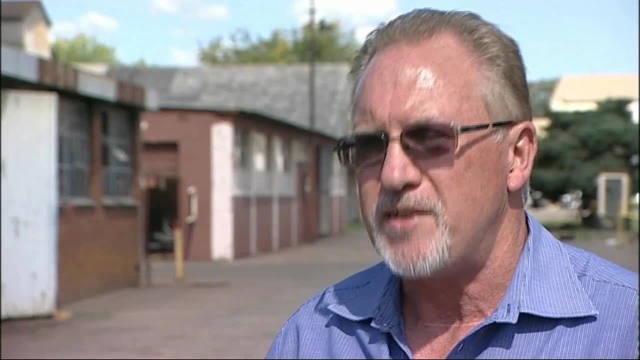 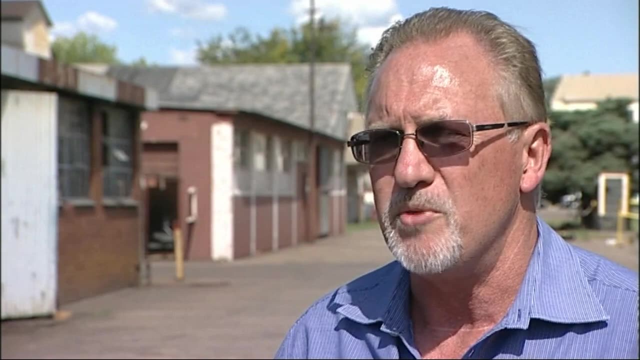 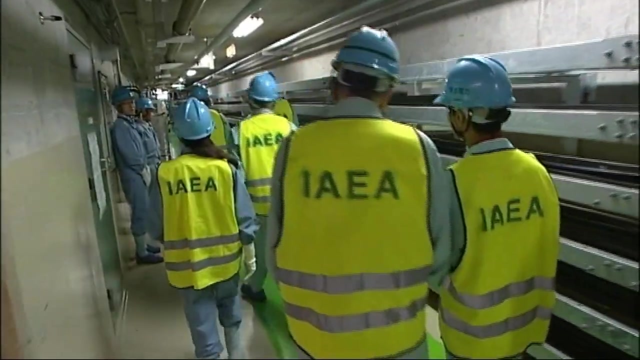 to do this as well. If the radiographer does not put safety first every single time that he's doing work, it can be a very big problem in terms of danger to himself and to members of the public, and can lead to disastrous consequences. Clearly, the agency cannot oversee the millions of applications. 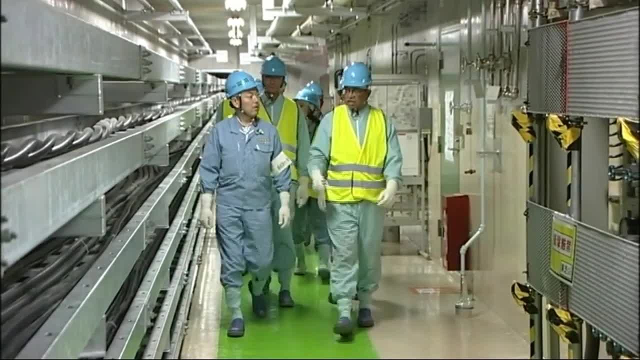 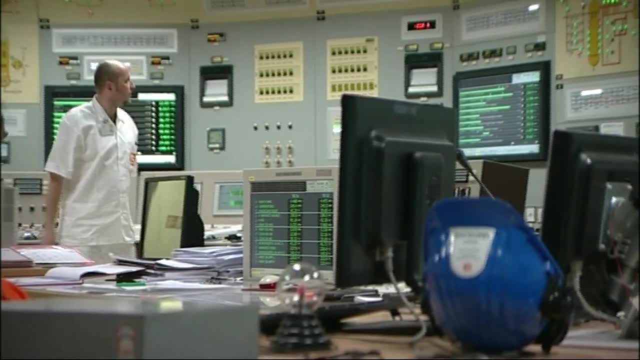 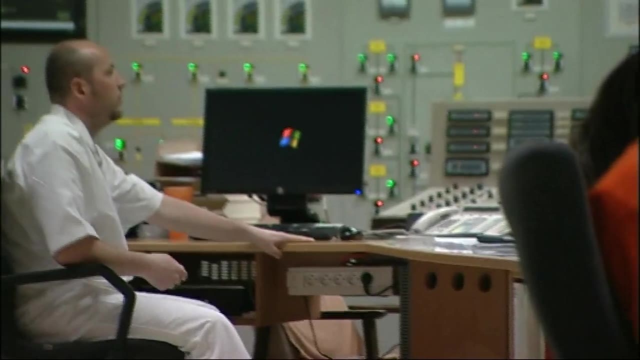 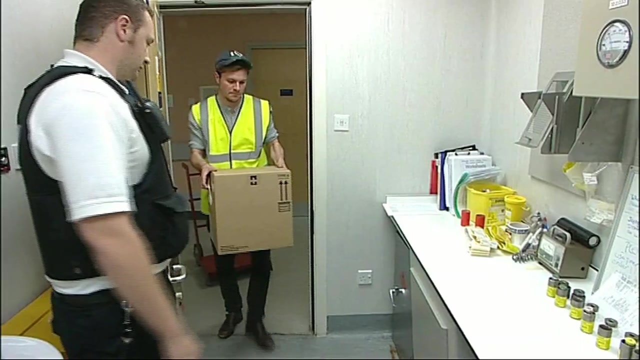 of ionising radiation that take place in workplaces all over the world every day. But, as well as establishing safety standards and guideline standards, its work in assessing and monitoring exposure, in education and training, in the establishment of information networks and systems, the IAEA does a great deal to encourage strict adherence. 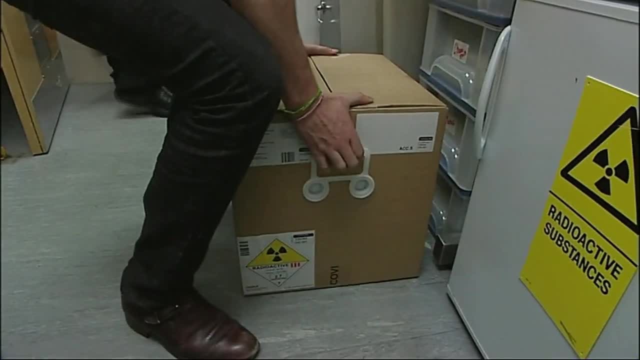 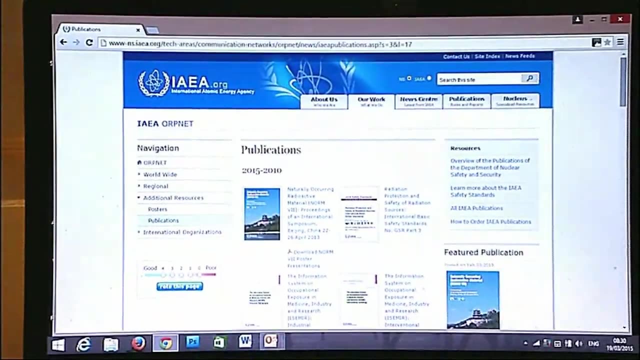 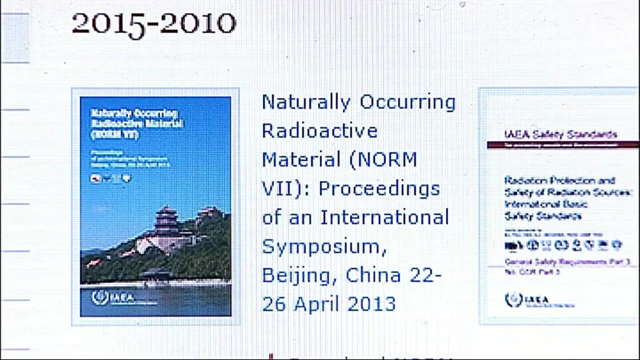 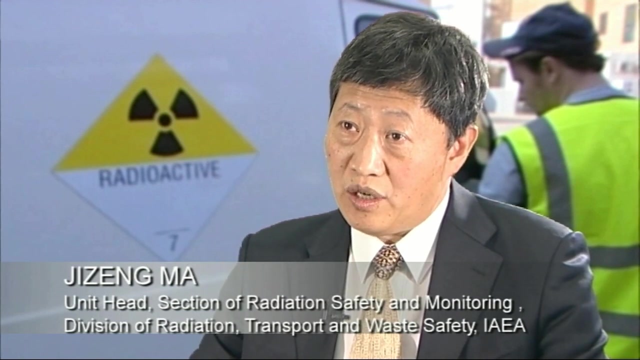 to the principles and practices set out in this film. The Radiation Safety and Monitoring Section has a very popular website where a great deal of information can be found and where educational materials can be downloaded For occupational radiation protection under the International Action Plan on Occupational Radiation Protection. 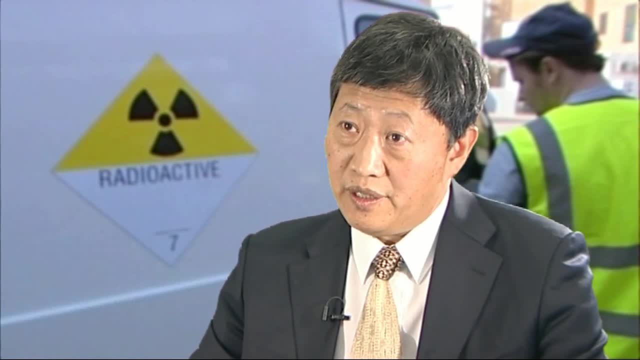 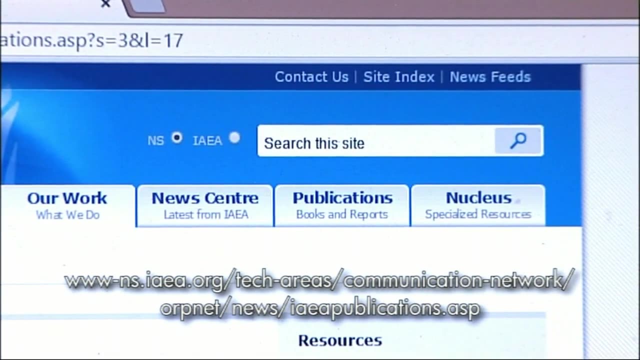 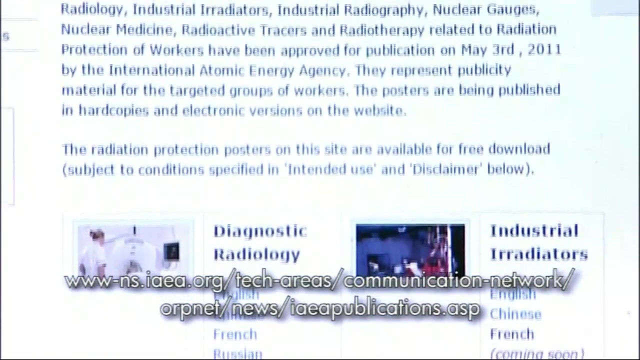 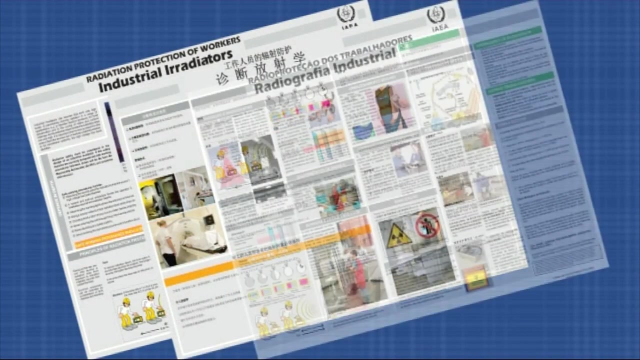 we created a web page. It's OFNET- Occupational Radiation Protection Networks, And the website is called. It's a focal point for occupational radiation protection and you can find all the information on occupational radiation protection on this web page. We prepare seven posters for protection of workers in different sectors. 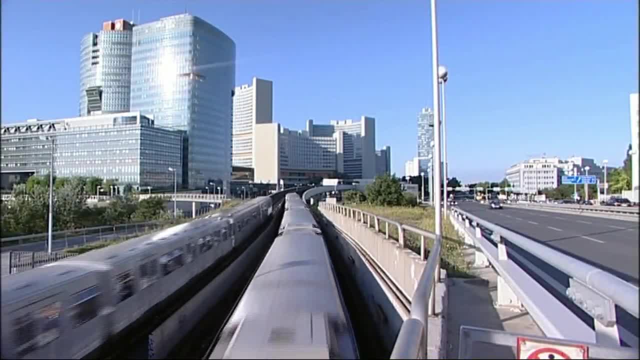 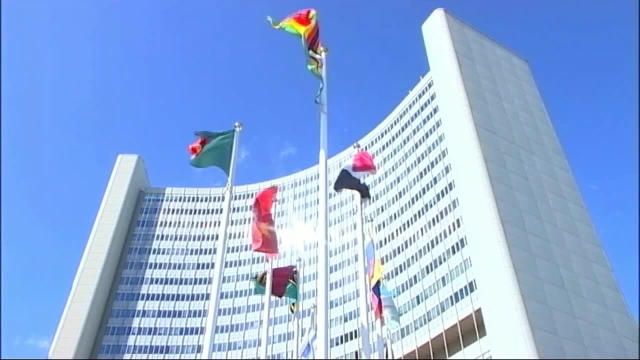 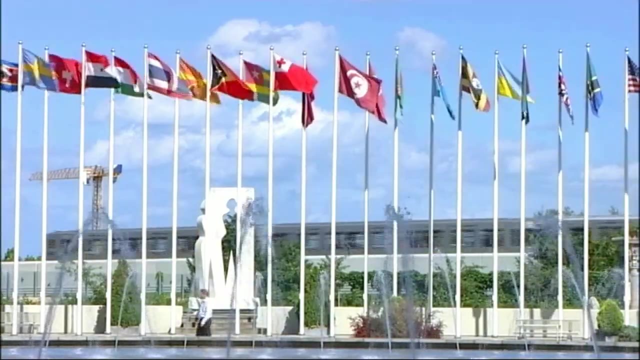 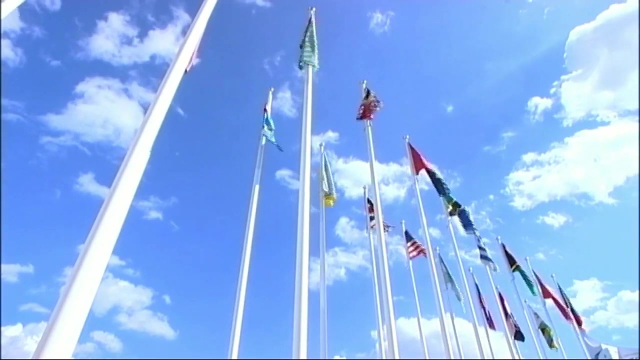 One of the most valuable services the IAEA provides is the Occupational Radiation Protection Appraisal Service. These provide an opportunity for Member States to have their Occupational Radiation Protection programmes independently assessed and evaluated. This is often useful to maintain or enhance the effectiveness of the programme. 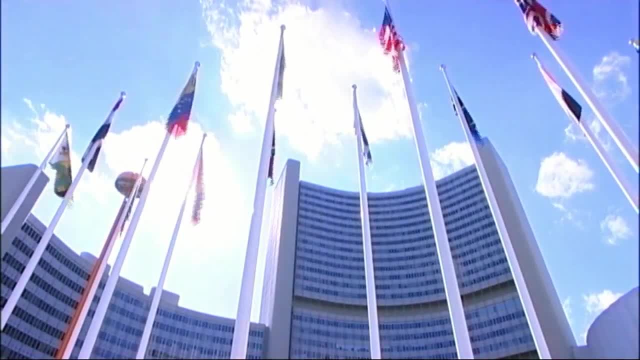 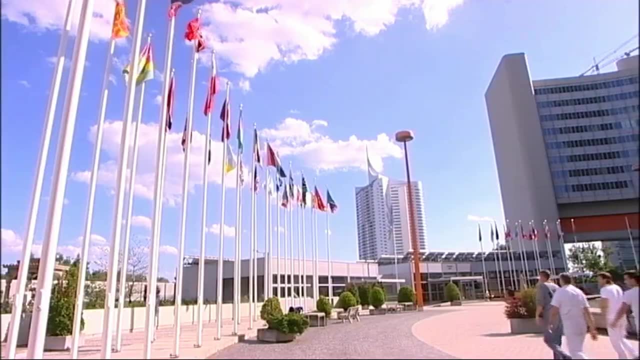 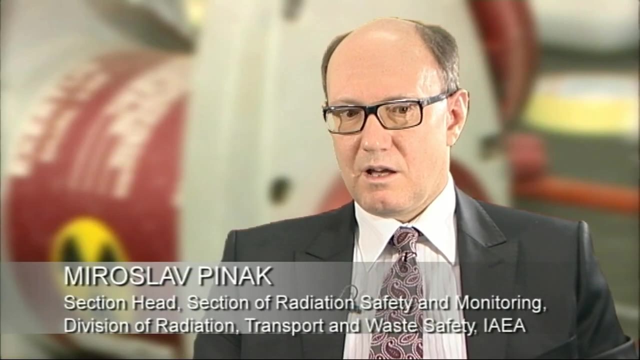 and to identify in an objective and unbiased manner the areas where improvements may be required. It also allows information on best practices from the host country to be made available to other Member States. Many countries are approaching the IAEA to ensure that the all-pass mission is being undertaken. 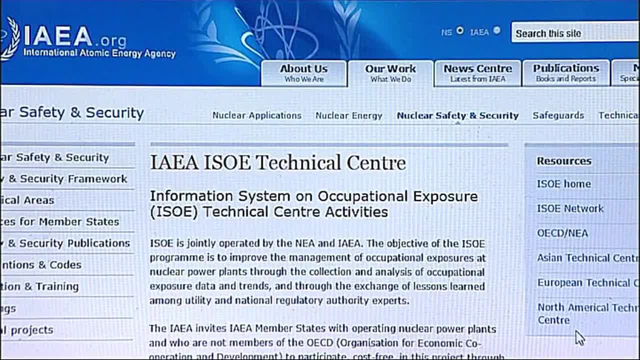 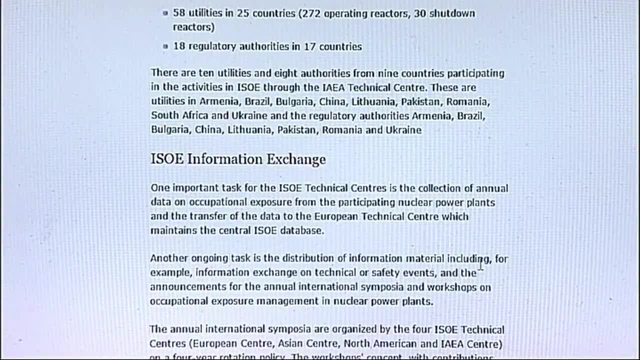 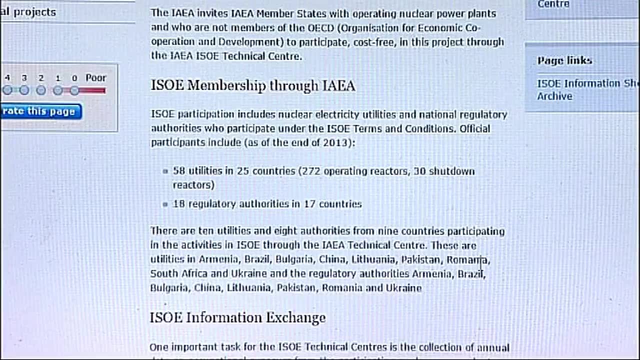 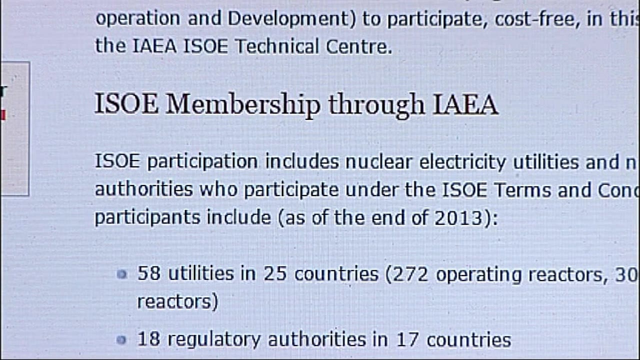 Another very popular service to Member States is the Information System on Occupational Exposure, or ISO. This is jointly operated by the IAEA and OECD Nuclear Energy Agency and provides broad and regularly updated information on methods to improve the protection of workers and on occupational exposure in nuclear power plants. 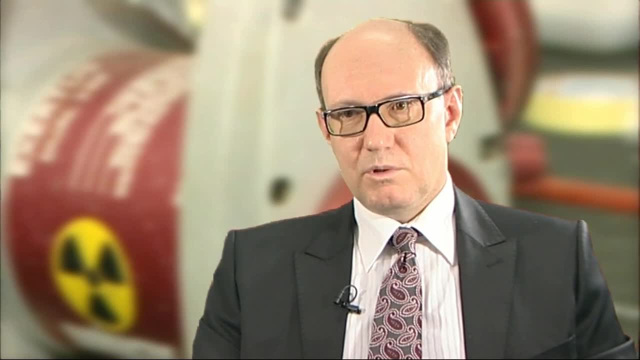 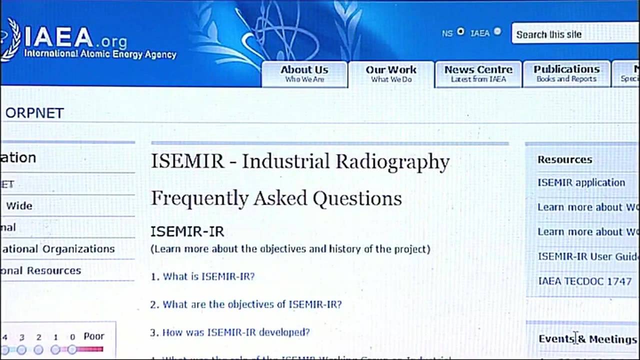 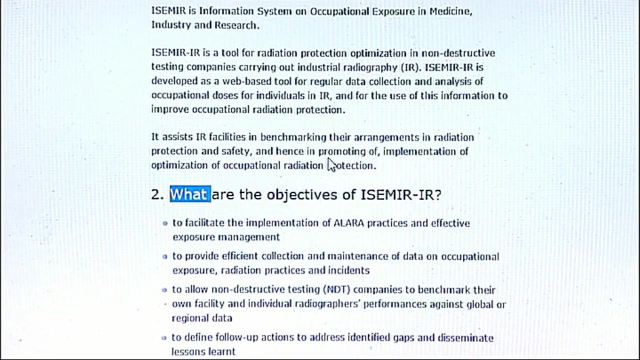 It ensures that good practice on Occupational Radiation Protection is shared about most nuclear power stations with operators. And yet another service is ISMIR, the Information System on Occupational Exposure in medicine, industry and research. ISMIR-IR is a tool for radiation protection optimisation. 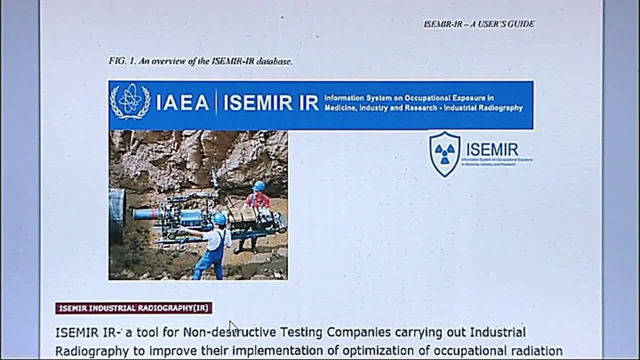 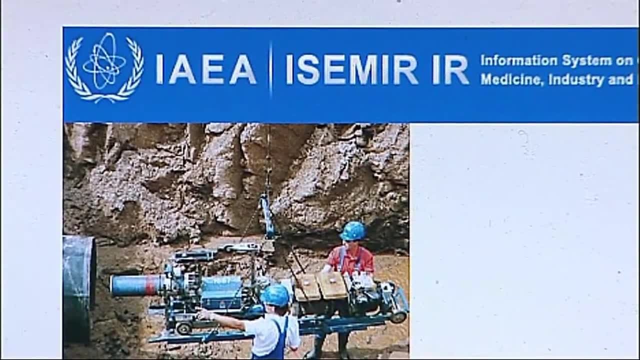 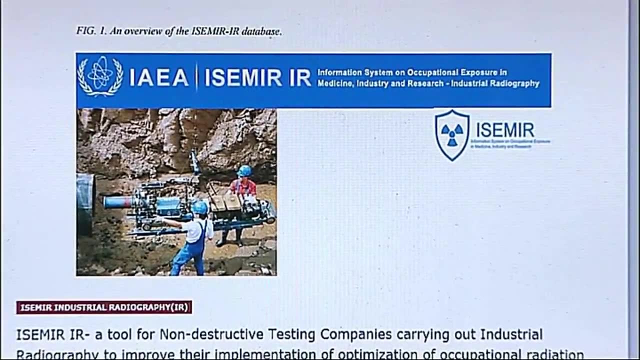 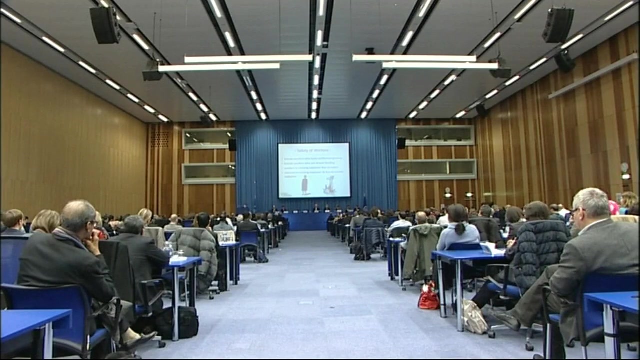 in non-destructive testing companies carrying out industrial radiography. ISMIR-IR is developed as a web-based tool for regular data collection and analysis of occupational doses for individuals in IR and for the use of this information to improve occupational radiation protection. ISMIR-IR is also used in the development